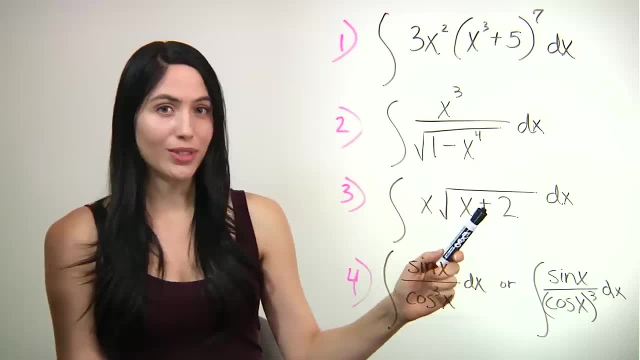 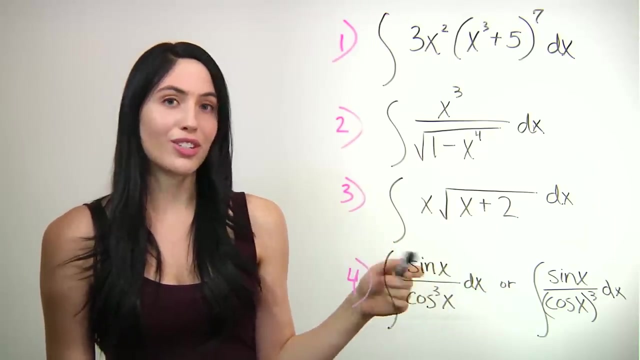 in your du. The third example has a square root in it and you'll have to manipulate the u-expression, rearrange the u-expression by subtracting a number in it in order to integrate easily. And the final type has trig functions in it and it's a fraction and you'll have to rearrange. 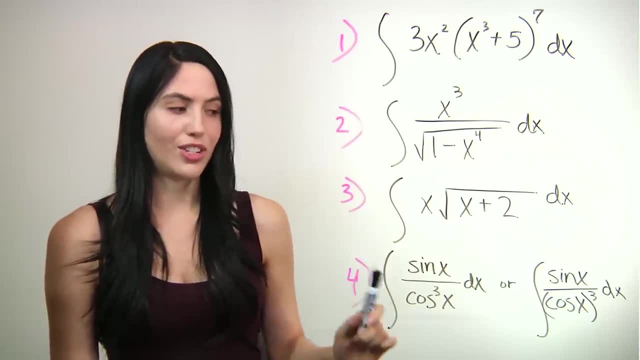 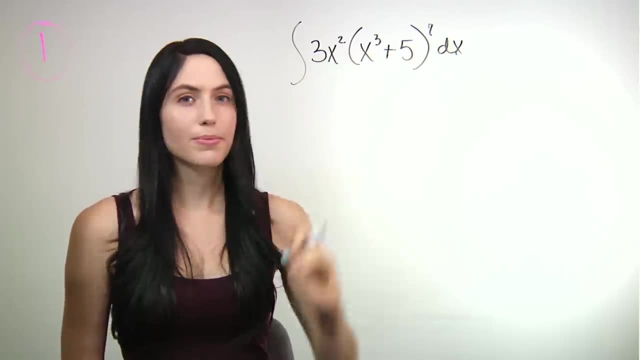 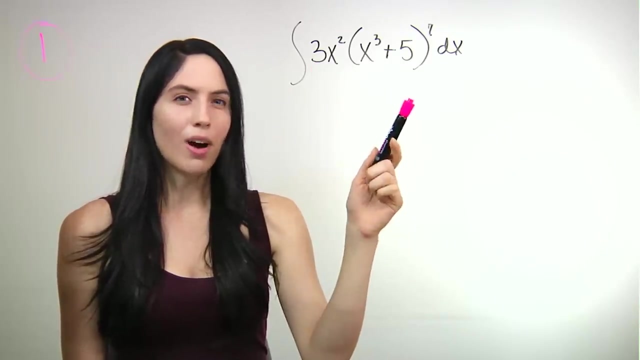 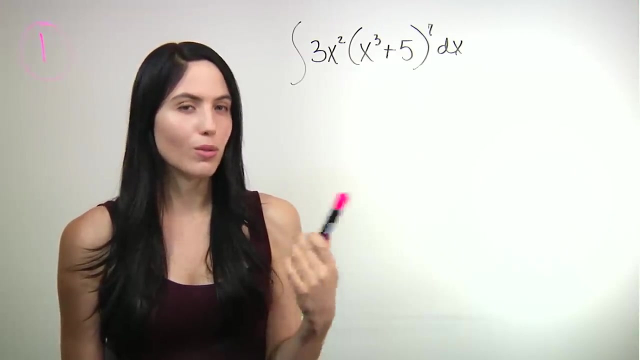 your du expression to integrate easily. Alright, so let's look at the first one. Alright, here's a simple example. Now, looking at this, I don't really know off-hand how to integrate that directly, but I can use a trick called u-substitution. Why is? 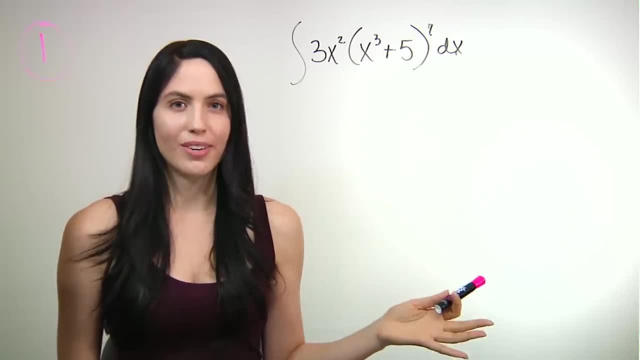 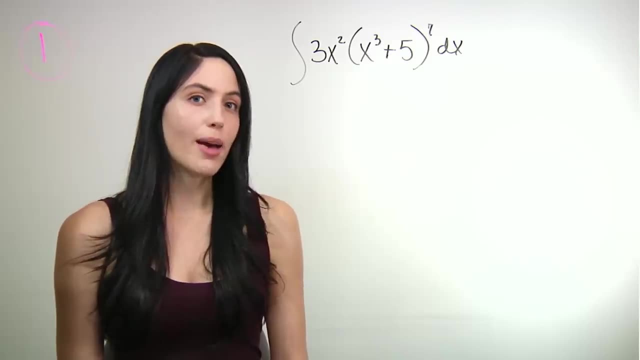 it called u-substitution. Well, no good reason as far as I know. They could have used any letter, but it's u. That's the standard, so we'll do u-substitution. and what that means is that you're going to rewrite this whole integral and we're going to have to do. 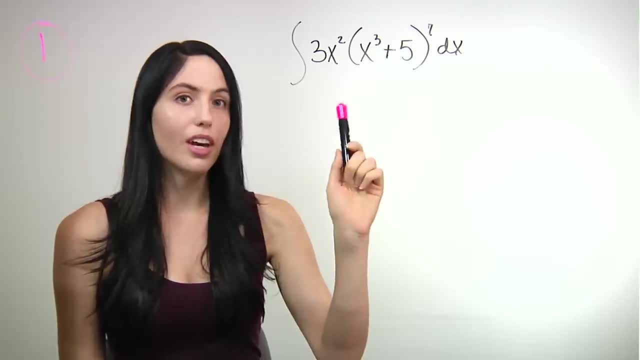 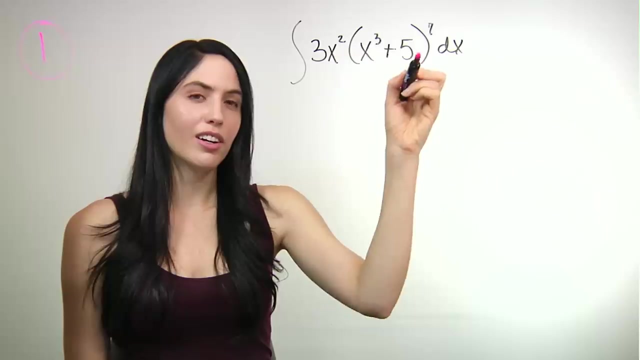 38.. in terms of the variable u, a new variable u. The first step is to pick your u expression. To pick your u expression, a good rule of thumb is that it's almost always the longer x expression that appears in the integral. 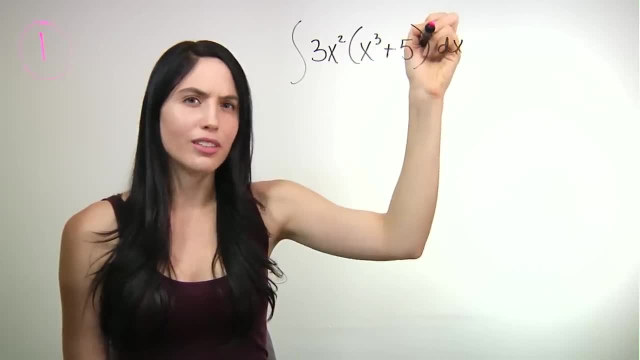 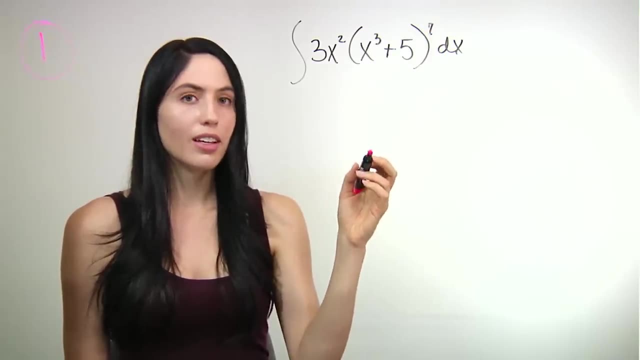 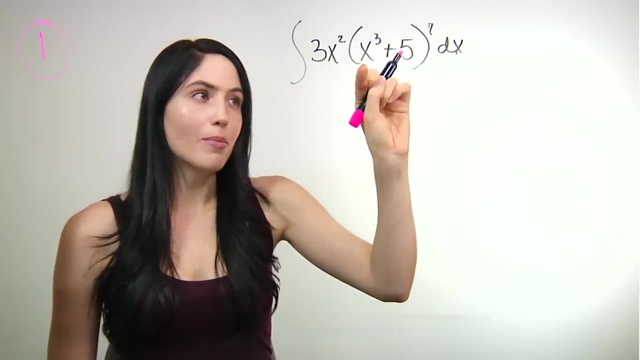 and the one that's inside some other function, inside some other form, like inside a power, inside a square root, inside the bottom of a fraction. What will always be true to use u substitution is that the integral will have some function and the other part will be the derivative of that function. 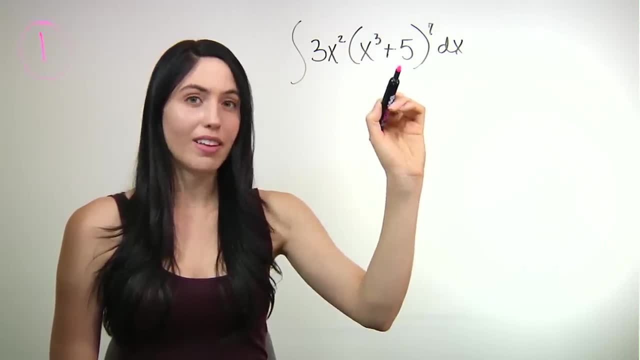 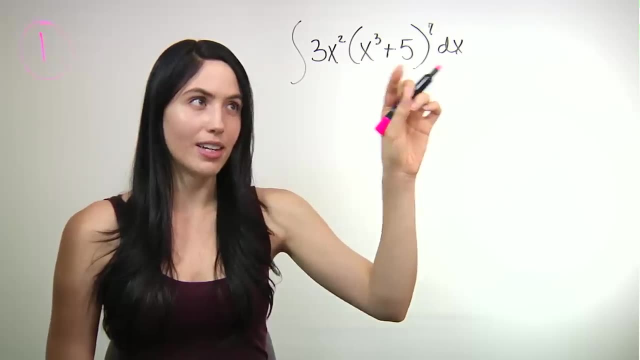 So notice that the derivative of x cubed plus 5 is just 3x squared, So you know that your u should be what's inside the parentheses here. Your u should be x cubed plus 5.. So go ahead and write that. 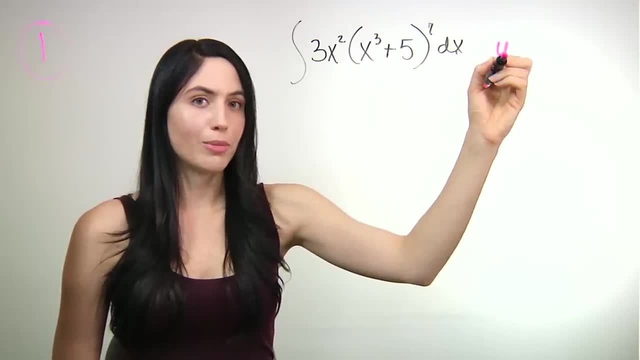 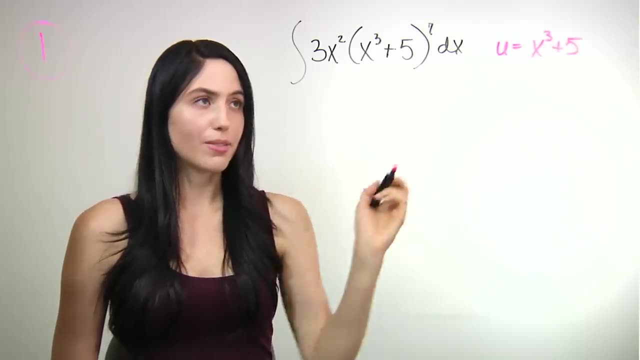 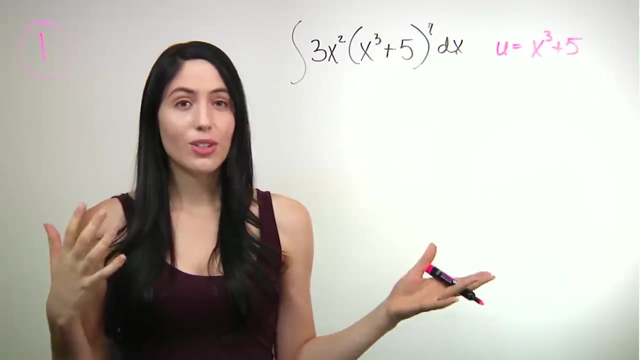 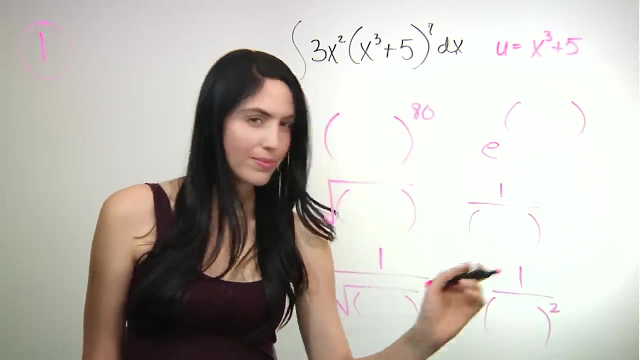 off to the side. You define your new variable, u, to be x cubed plus 5.. So say, you still don't know how to pick your u expression? Yeah, it's not obvious, It's kind of tricky. So let me show you another way of thinking about it. 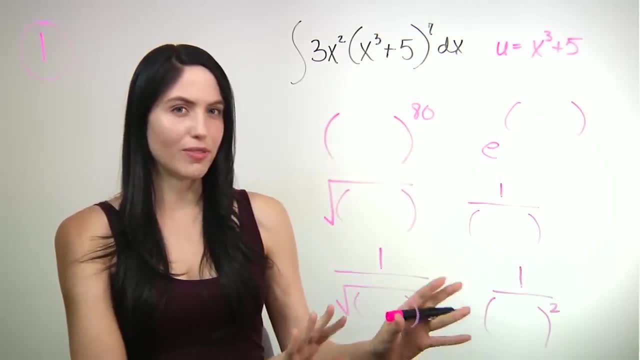 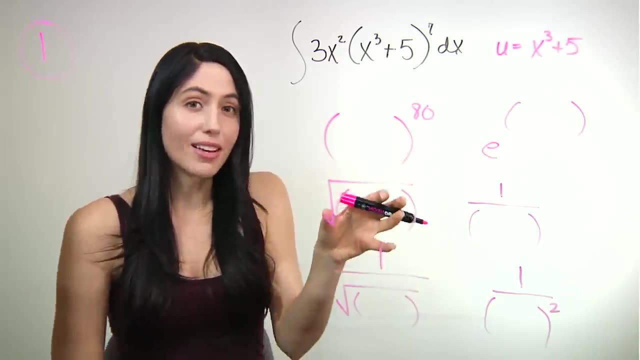 Okay, so look at all these forms that I drew, these function forms. You could have something to a power e raised to something, something under a root, something in the bottom of a fraction, something in the bottom of a fraction and under a root. 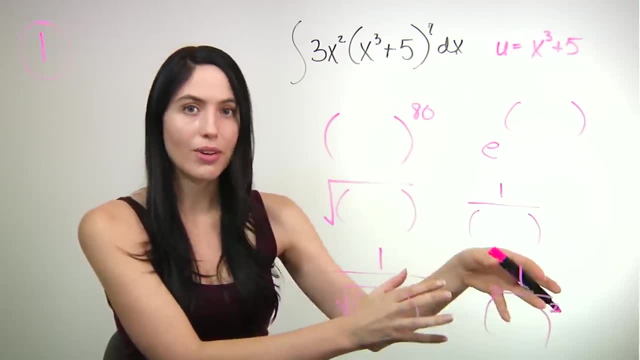 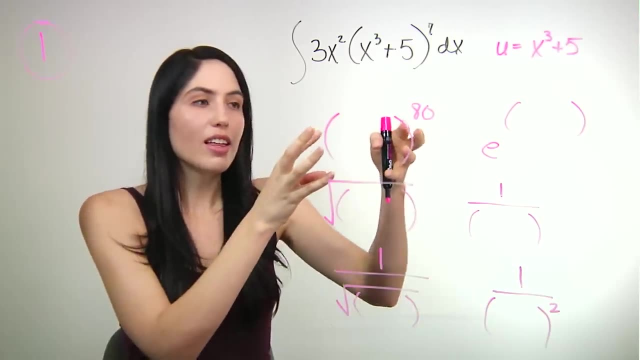 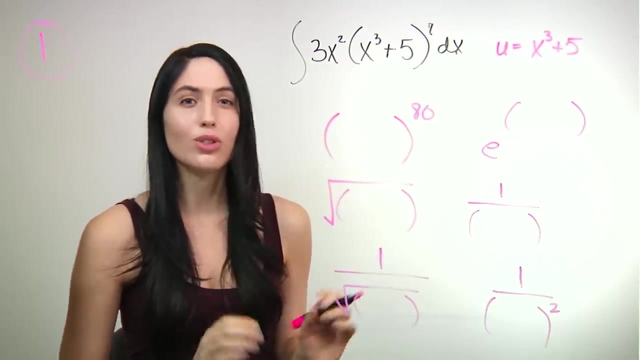 and something in the bottom of a fraction and raised to a power in the bottom, No matter what it is. any of these forms, the thing that is inside another function in parentheses- is almost certainly your u expression. It's what you should define as your u equals. 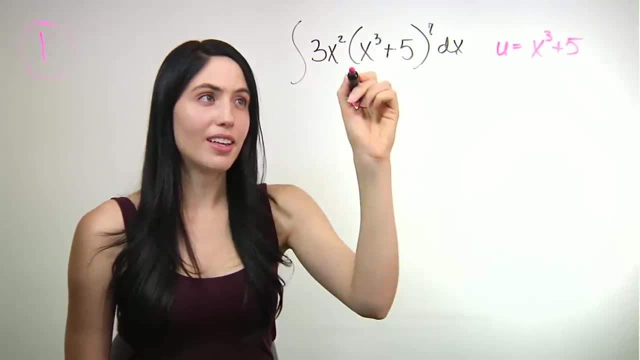 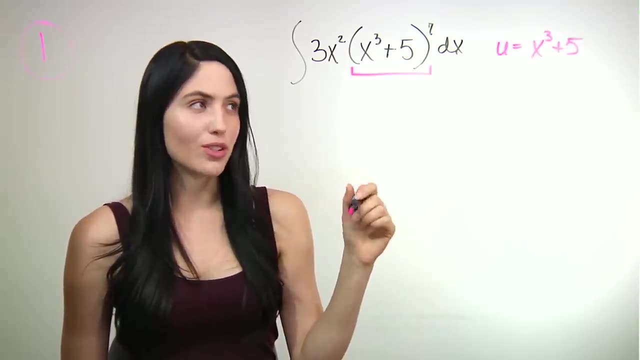 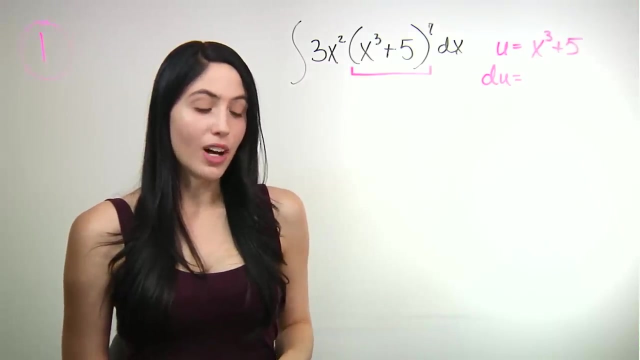 Okay, so you found your u, x cubed plus 5. This is your u. The next step is to find du. the differential du equals to find du. all you do is take the derivative of this side with respect to x. 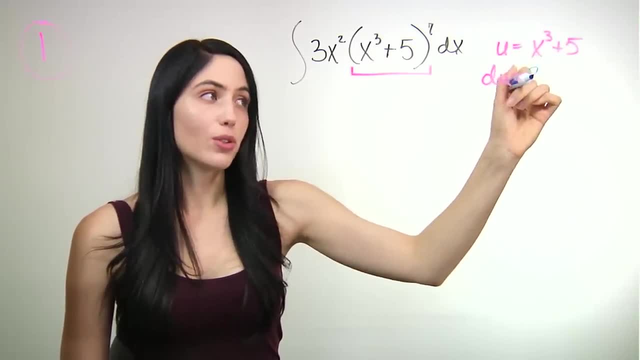 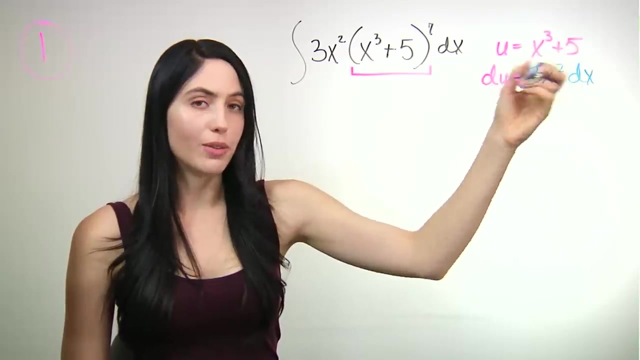 So, as you know, what that should give you is 3x squared plus nothing, since 5 is a constant, And what you have to write at the end of your du- differential- is a dx, always, because you took the derivative with respect to x. 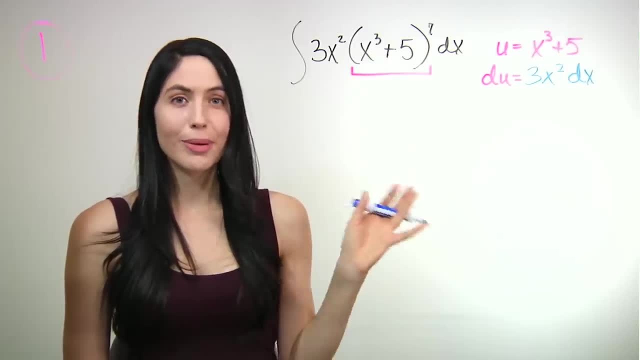 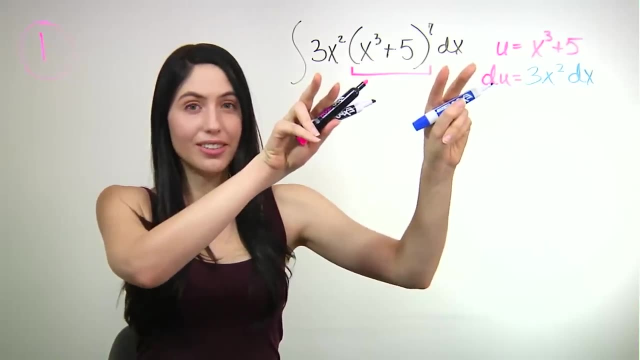 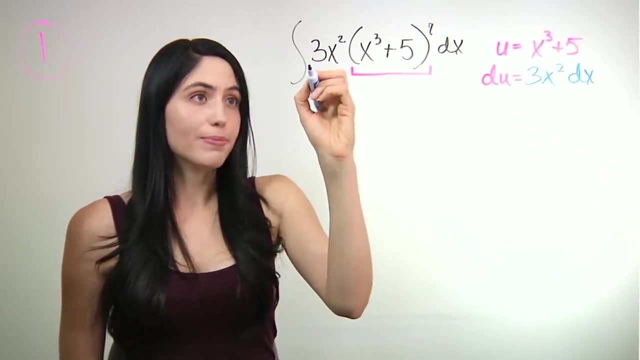 Now, in a perfect world, perfect problem, your du 3x squared dx is exactly what's left in the integral apart from u, And this is a simple, perfect world problem. So it is This part 3x squared, what's left. 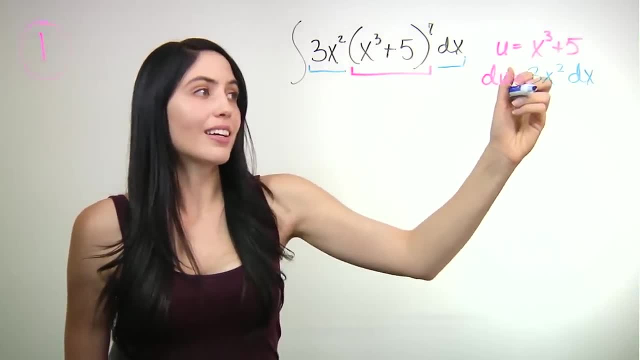 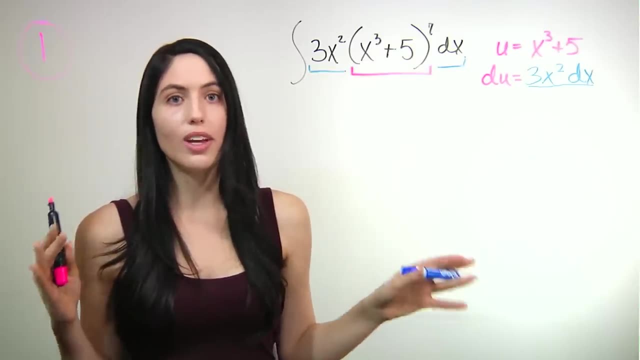 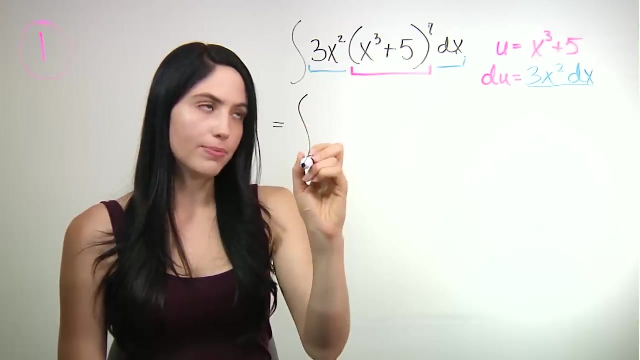 3x squared dx is exactly your du. What this means is that you're ready to substitute and get everything completely in terms of u and du, So let's do that In the next line of work. you have an integral of. 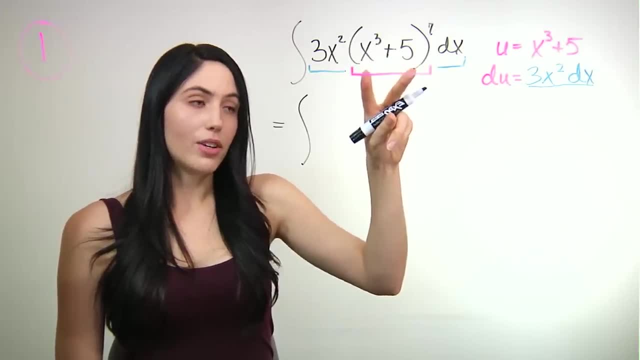 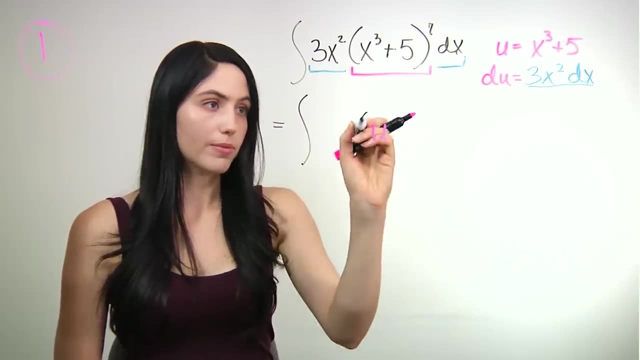 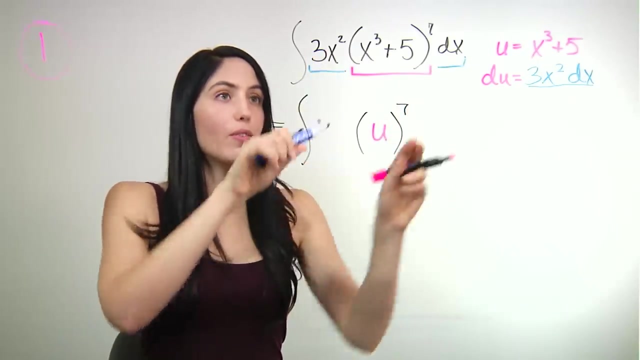 remember. in place of xq plus 5,, you're writing u, This is u to the 7th power, And in place of 3x, in place of 3x squared dx, you're writing simply du, because what's left? 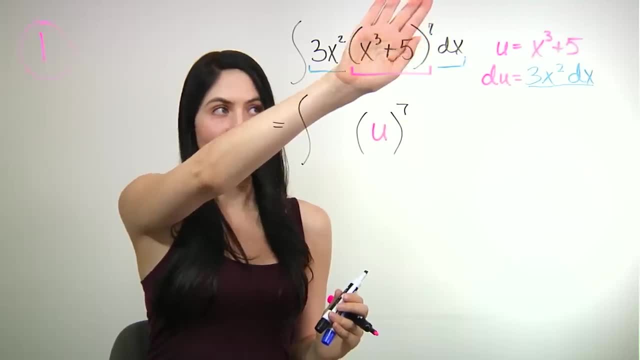 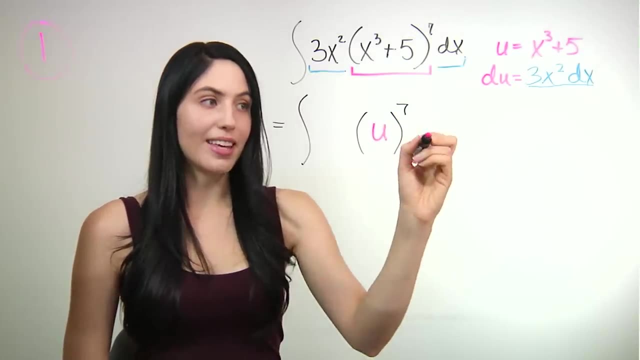 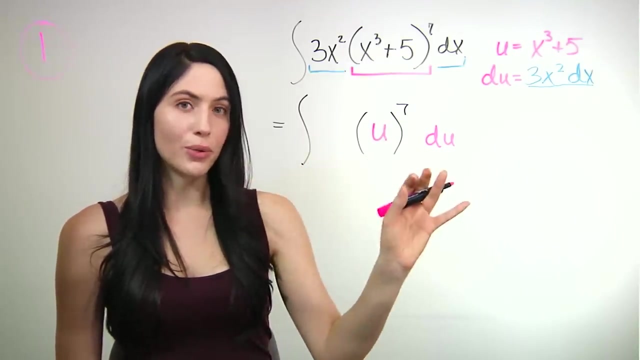 after you take that away is just 3x squared dx. So you put in place of that du. The du always goes at the end of your integral, not in the front. So this is now your integral, all in terms of u du. 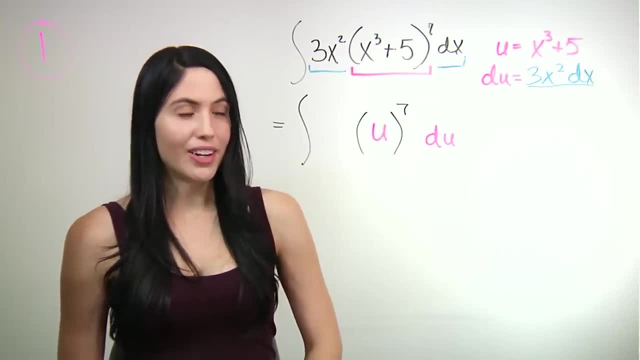 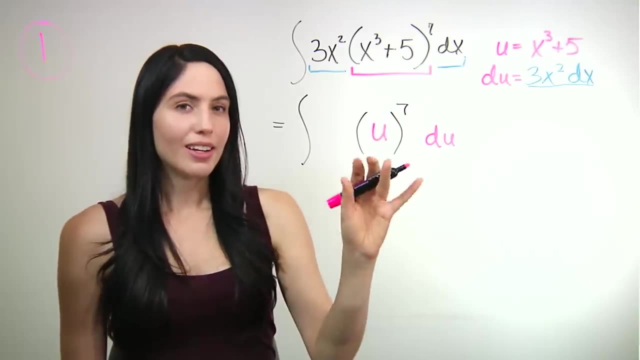 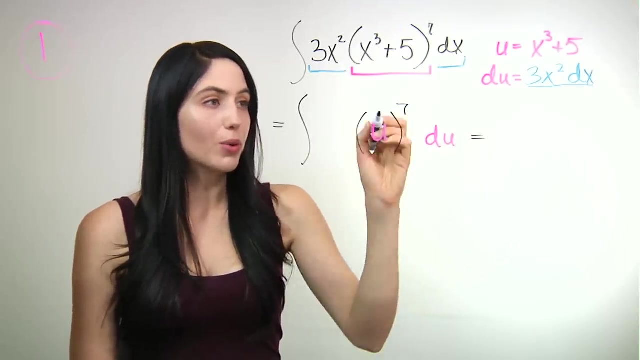 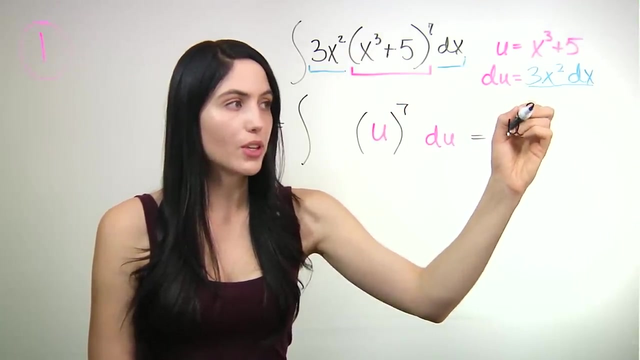 This should look like something you know how to integrate, because it's just a variable raised to power. You use the power rule. If you don't remember how to do that, the pattern is to raise this power by 1, so it becomes u to the 8th. 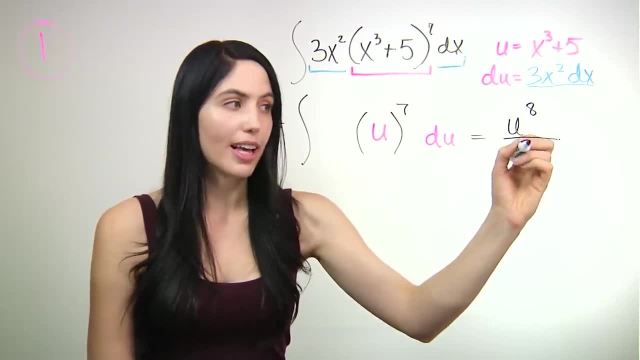 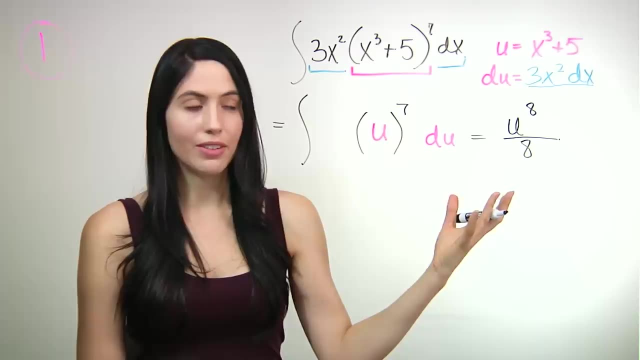 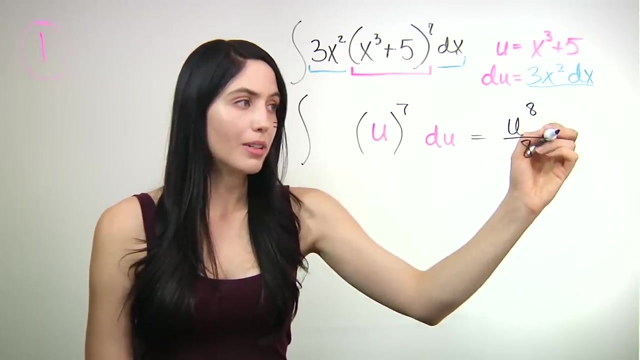 and divide by that new power 8.. And since this is an indefinite integral, indefinite antiderivative, meaning there are no limits- you have to write at the end plus c. Don't forget that. Plus c, Alright, you've integrated. 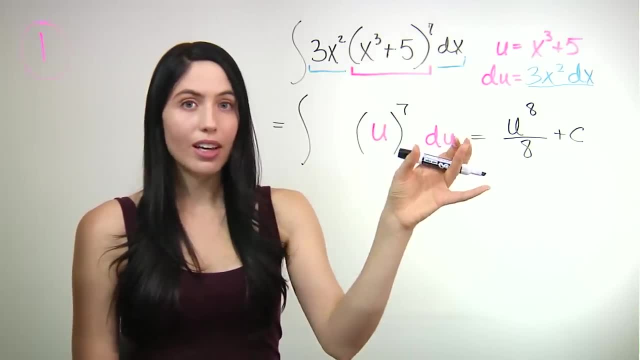 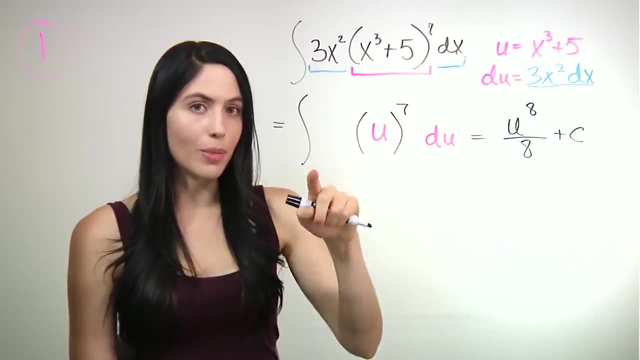 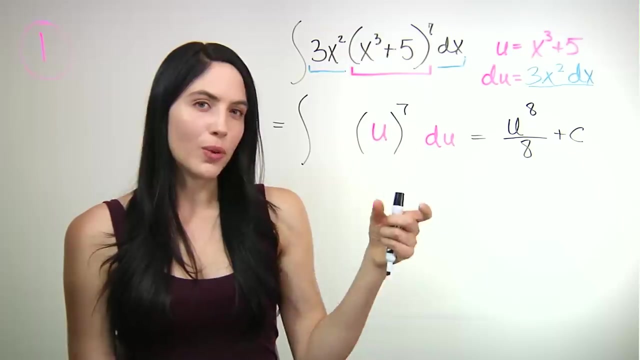 What happened to the du? It does just disappear when you integrate. When the integral sign, the integral symbol goes away, so does the du. You can think of it as undoing the chain rule, the inverse of the chain rule. The du just drops out. 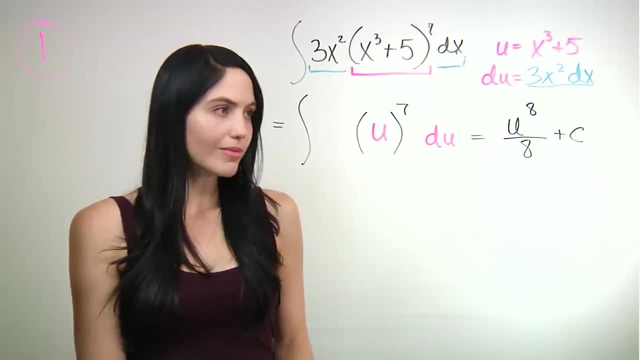 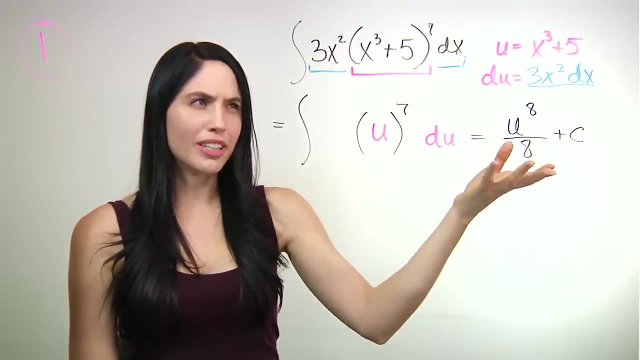 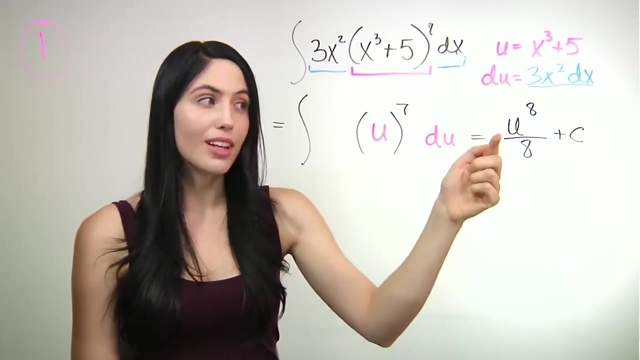 It goes away. So it goes away. Now you've integrated, You've evaluated that integral, But what you were originally given was in terms of x, not u. So there's another step where you have to back, substitute and plug in. 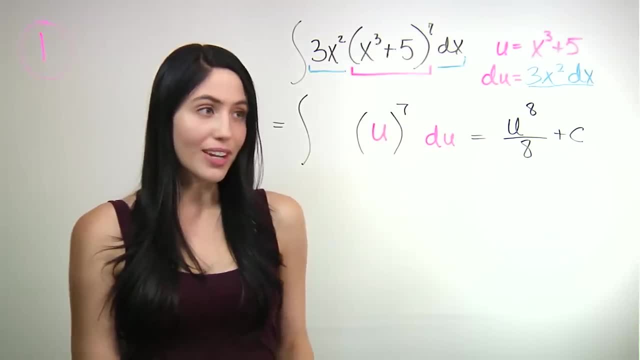 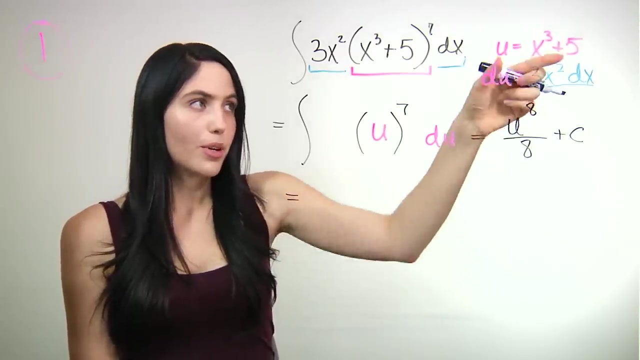 for what u originally was. Notice that your? u substitution made it very easy to integrate. That was the whole point of substituting. But now the final step: In place of? u you want to back, substitute, put in for u what you defined it to be. 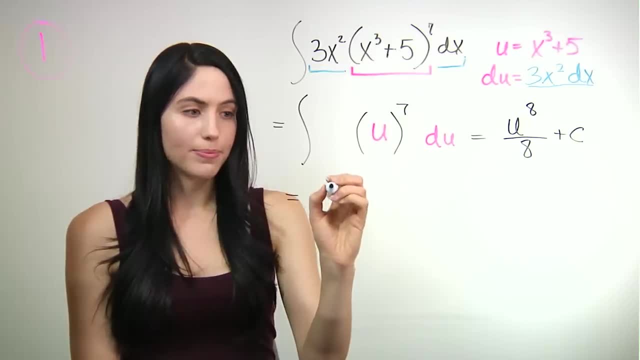 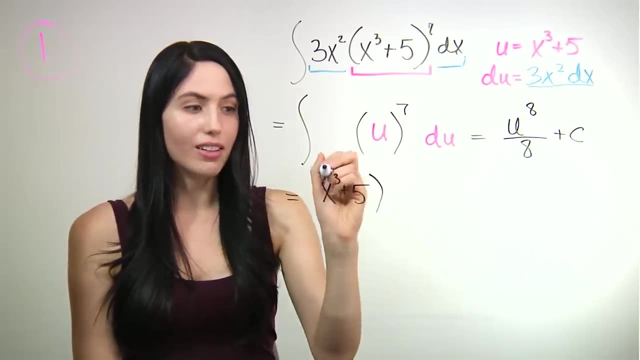 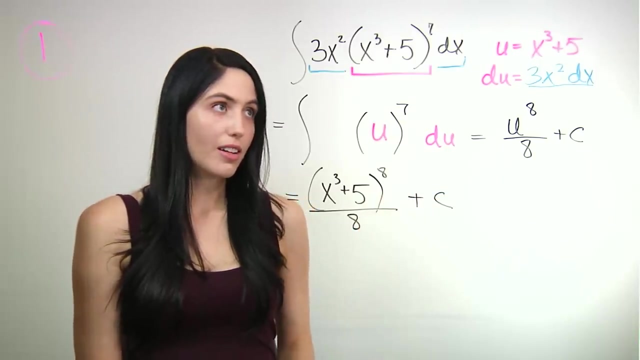 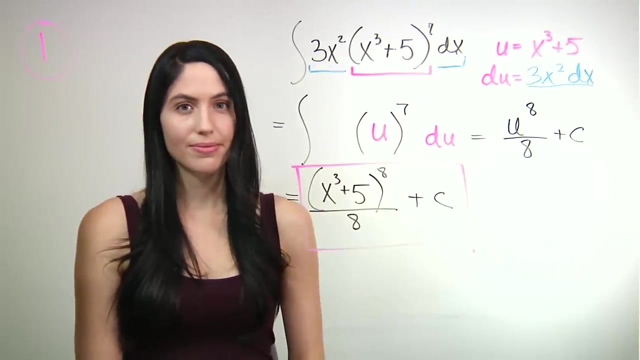 x cubed plus 5.. So we have x cubed plus 5 to the 8th power. It's all to the 8th power over 8 plus c. So that is your final answer for the integral Sometimes. 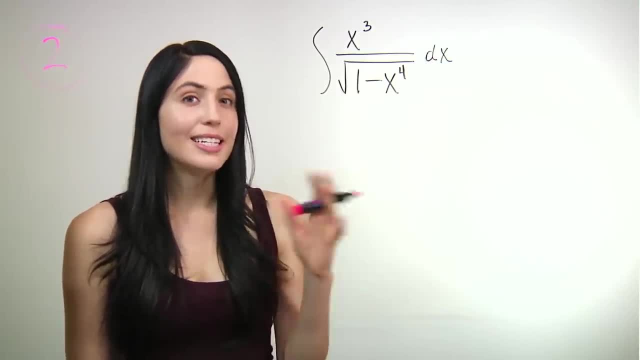 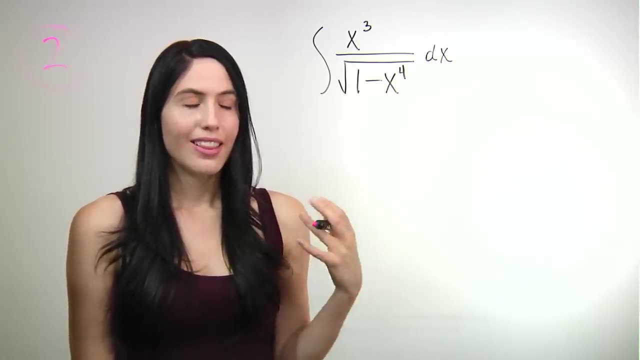 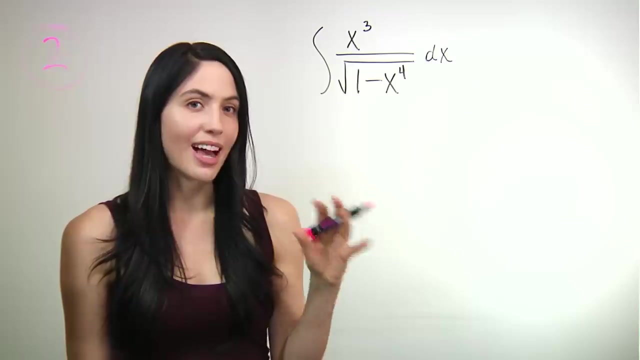 when you pick a? u expression, the du, the derivative you get does not give you exactly what you need to integrate right away. Then what you have to do is manipulate the du or the? u, Rearrange it so you have exactly what you need. 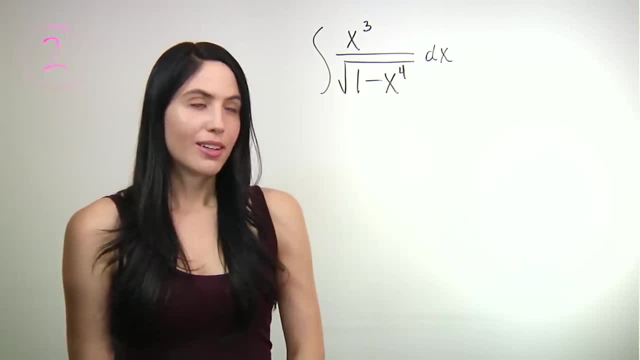 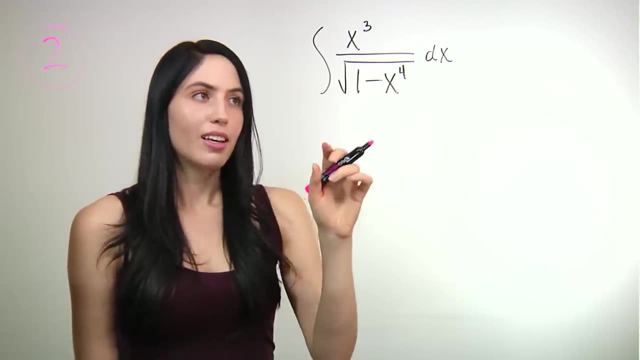 to make the substitution work out. So let's try this example. Start the same way. You need to pick your u and pick it wisely. Think back to what I said about the forms. u is usually the longer x expression, that's inside. 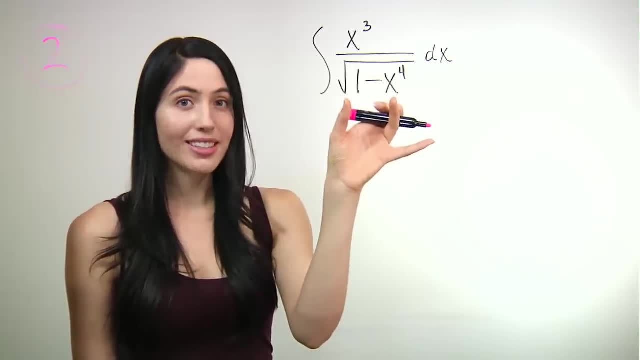 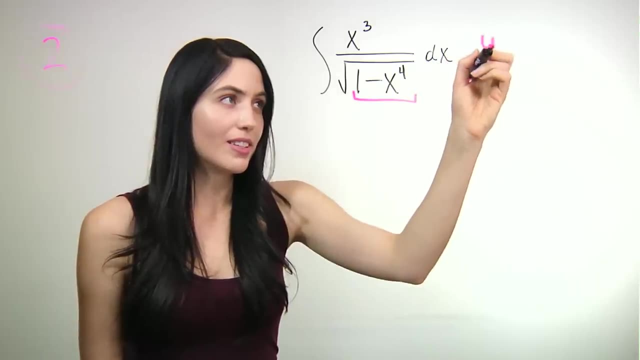 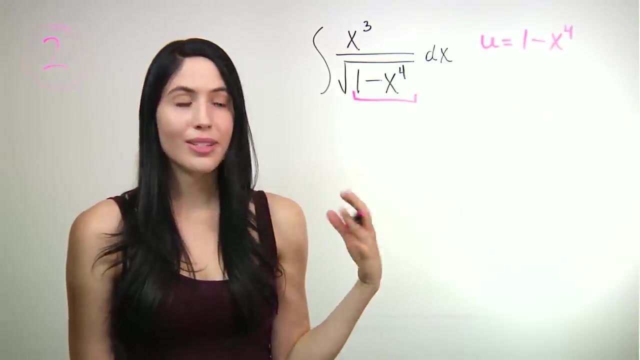 another function form. So a good choice would be 1 minus x to the 4th. So right off to the side, u equals 1 minus x to the 4th. If you're wrong you can always go back. 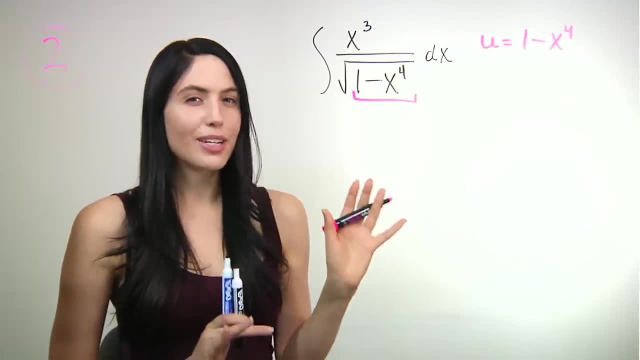 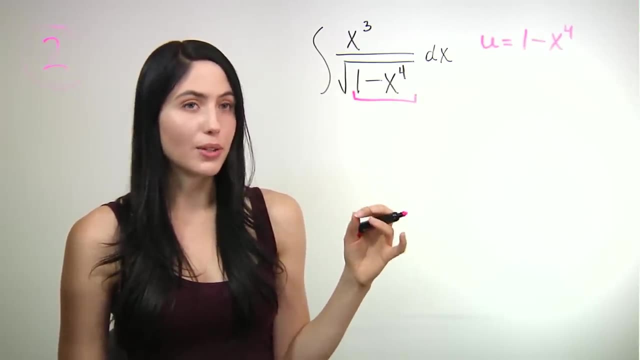 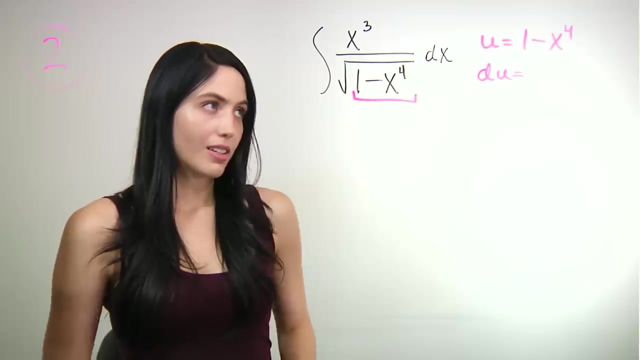 and pick a different u, But try to pick your best, what you think is the best option. Next step is to find the differential du du you get by taking the derivative of this expression with respect to x. So the derivative of the 1. 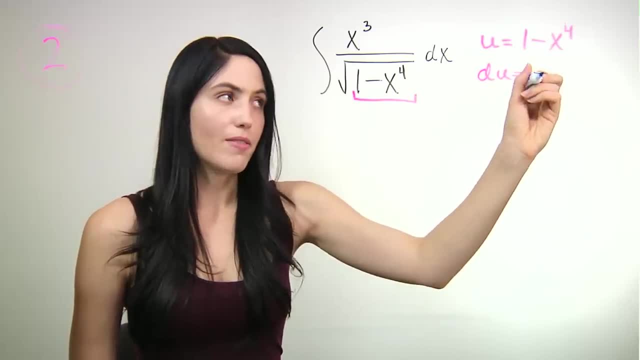 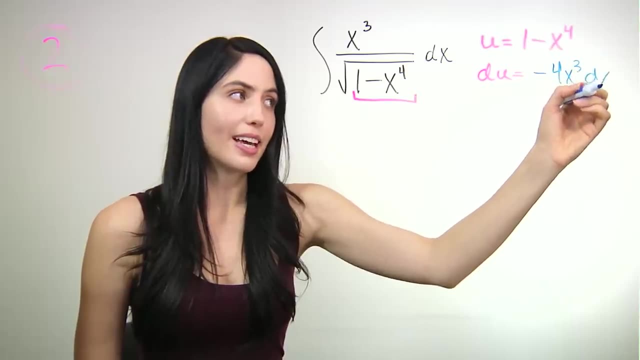 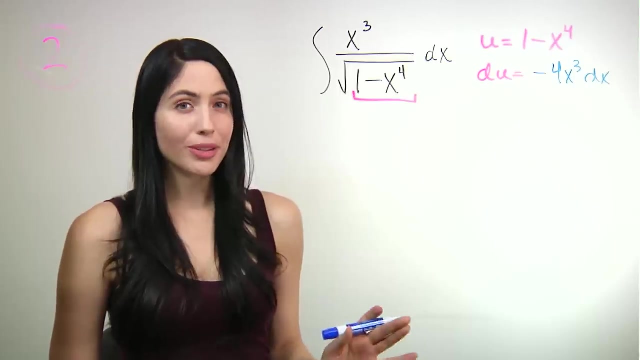 gives you nothing And in this part the derivative would be negative: 4 x cubed dx. Don't forget the dx. That's there because you took the derivative with respect to x. Okay, ideally, in a perfect world, this du. 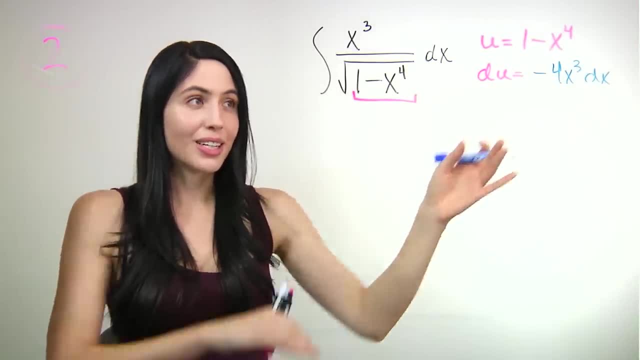 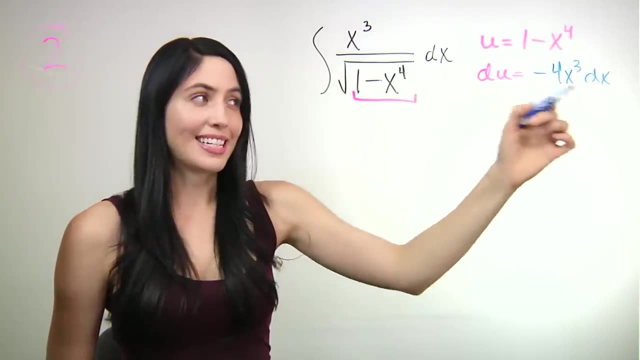 that you found would match exactly what you have left over in your integral x cubed dx. Unfortunately it doesn't. You have this negative 4 there that you don't want. Your job is to make it match up so that you can. 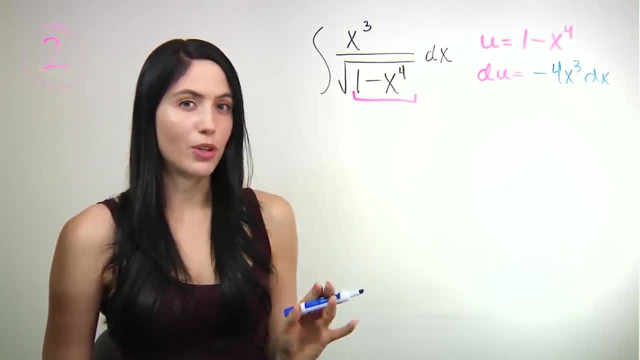 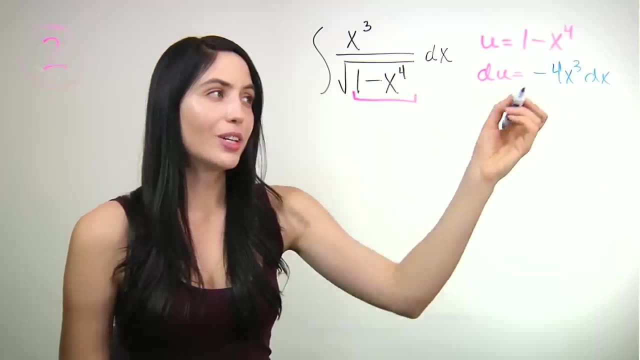 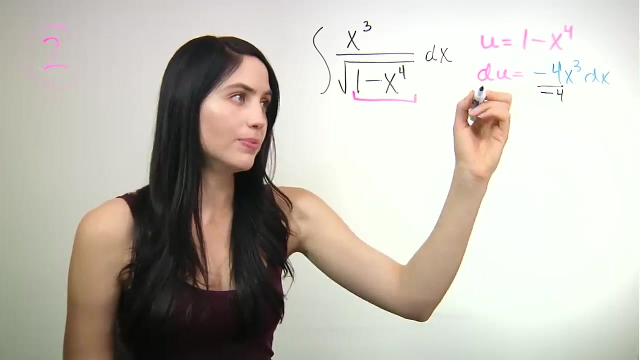 plug in here and get everything in terms of u and du. All you need to do is get rid of the number that you don't want. You don't want the negative sign or the 4.. So divide out negative 4 from both sides. 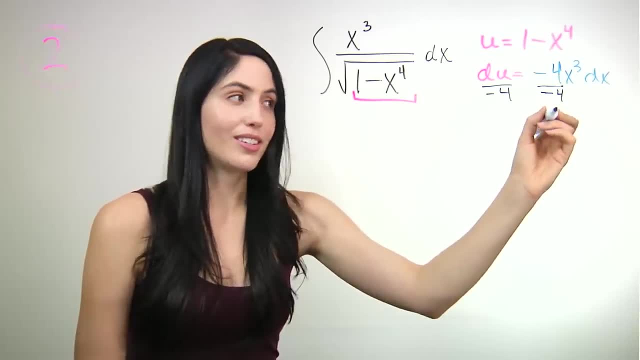 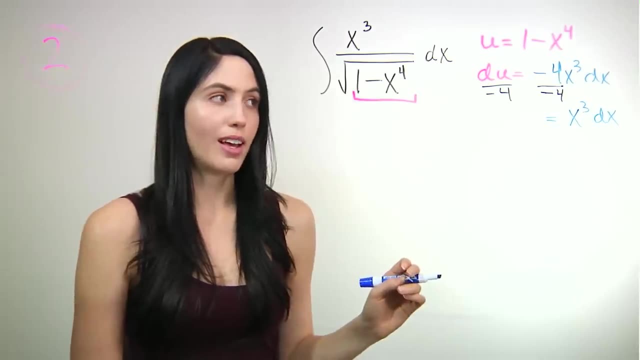 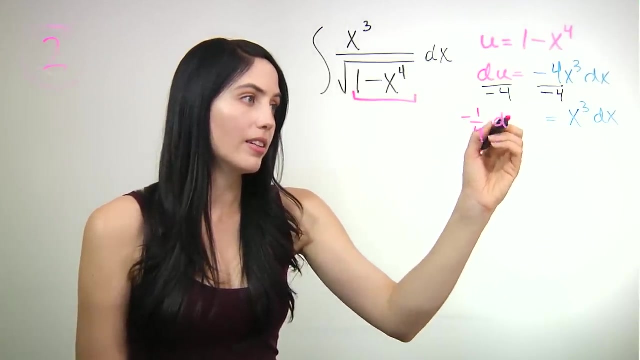 And what you have left over is what you want: just x cubed dx on one side, and on the other side you have negative 1 fourth du. Now you're ready to do the next step: to substitute everything in terms of u and du. 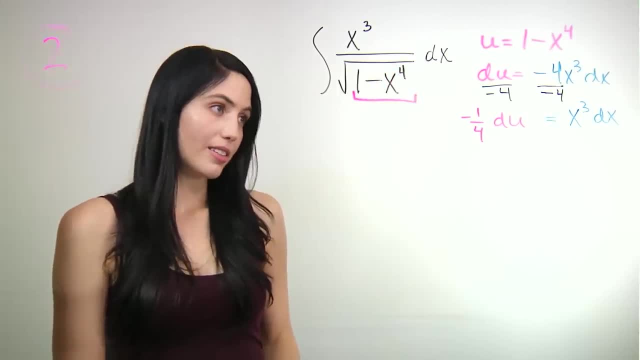 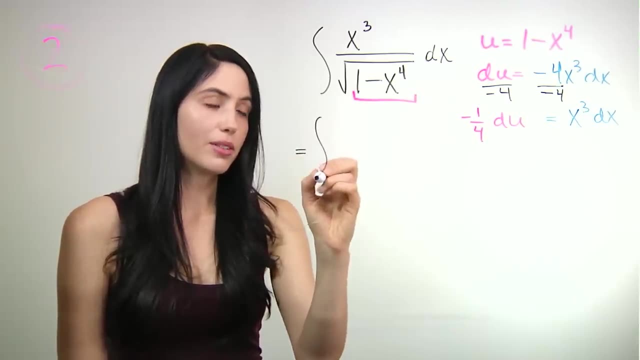 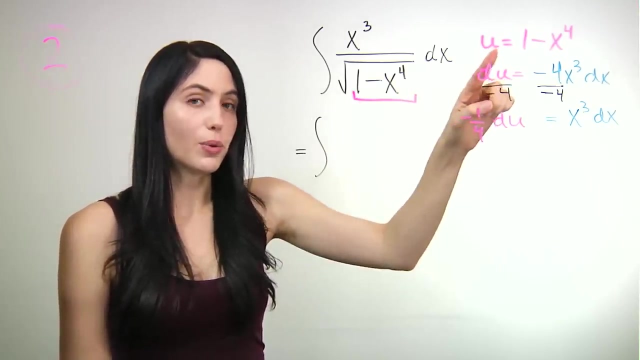 So let's rewrite that In the next line of work you'll have equals integral in place of 1 minus x to the 4th. you have just 1 minus x to the 4th, plus you have just u. So 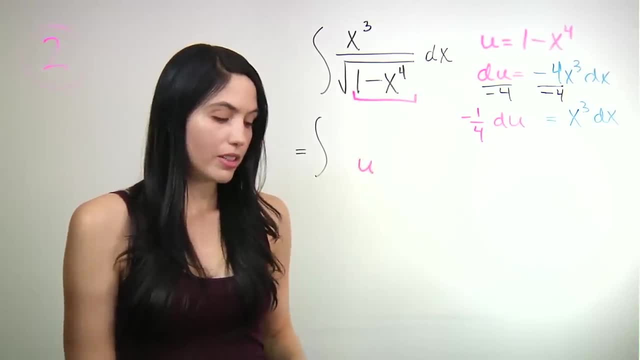 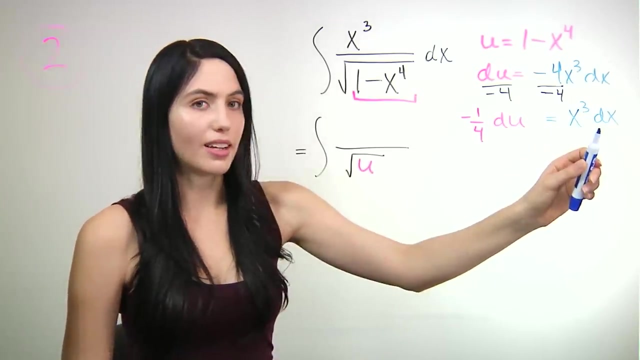 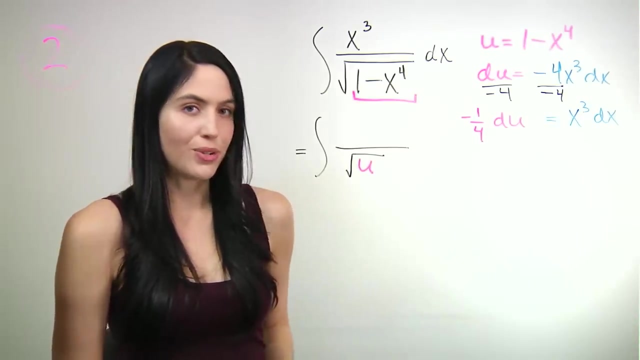 in the bottom you have a square root of u And then, in place of x cubed dx, in place of x cubed dx, you're going to insert: put in negative 1, fourth du, And you can just write that on the top. 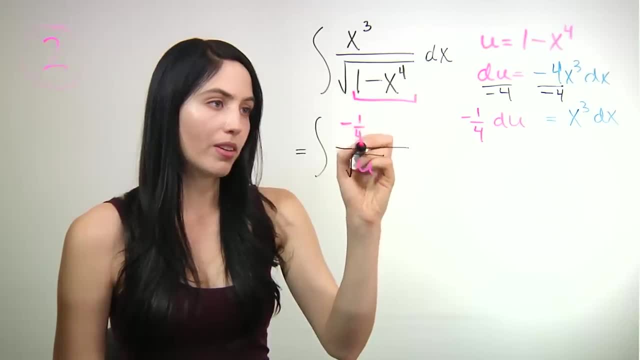 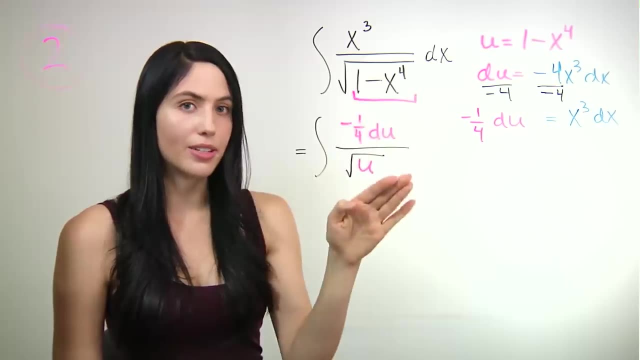 for now. Negative 1. fourth du: You don't need the dx anymore. You have a du now, because everything in this integral is written in terms of u and du. That's good, That's what you want, because it'll be easier for you to integrate now. 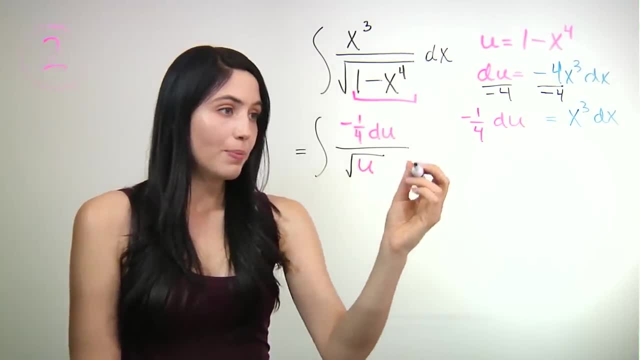 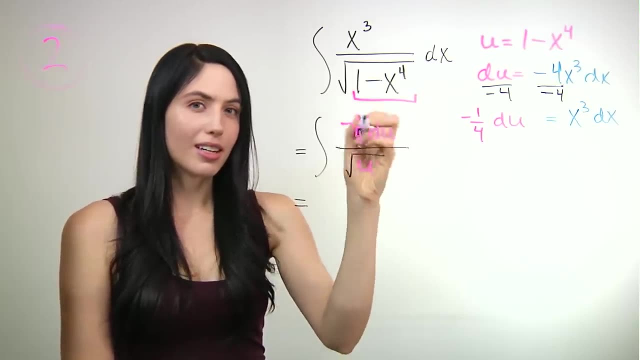 Let's do some simplifying In the next line. go ahead and pull that constant, the negative 1 fourth, out front. Negative 1 fourth integral. Any number, including the negative side, can be pulled out front and it will be easier to see. 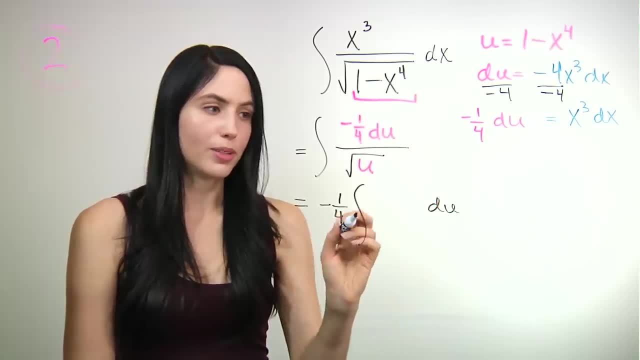 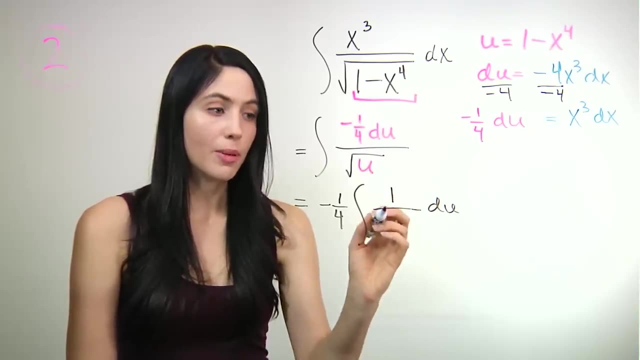 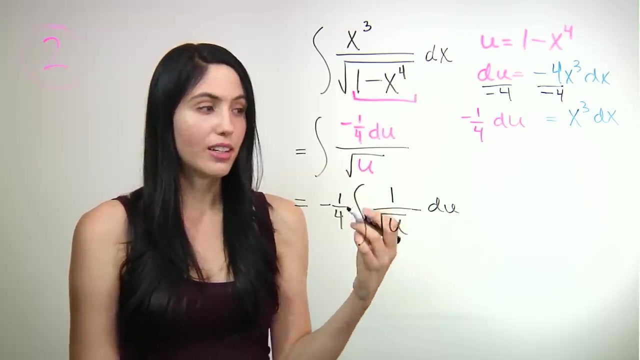 how to integrate. Leave the du at the end, as you normally do, So you just have 1, nothing but 1. on top and on the bottom you have a square root of u. This is more and more to integrate. Let's make it. 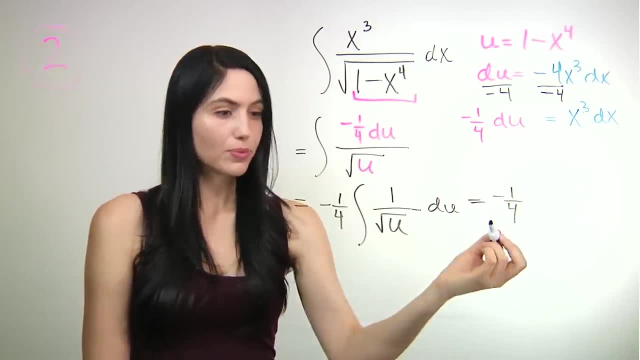 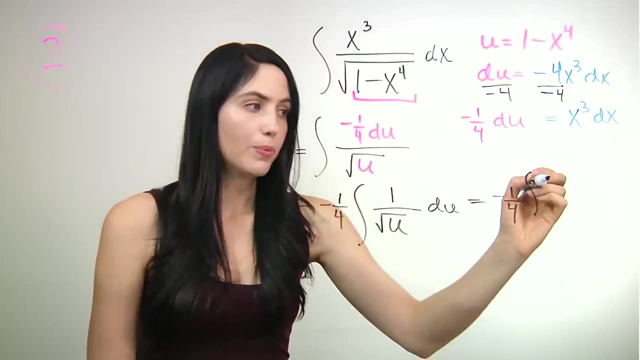 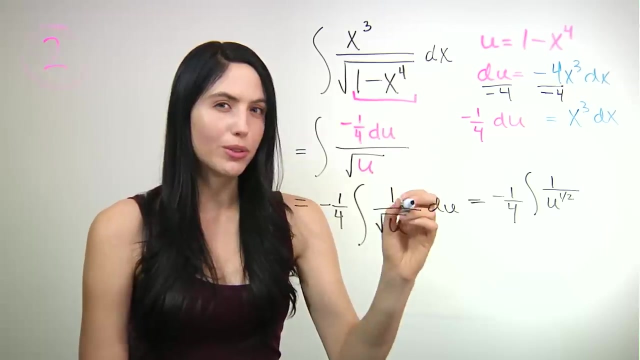 a little clearer, even more clearer. So you have negative 1. fourth integral: 1 over square root of u is 1 over u to the 1 half power. The square root of a variable can also be written as a variable to the. 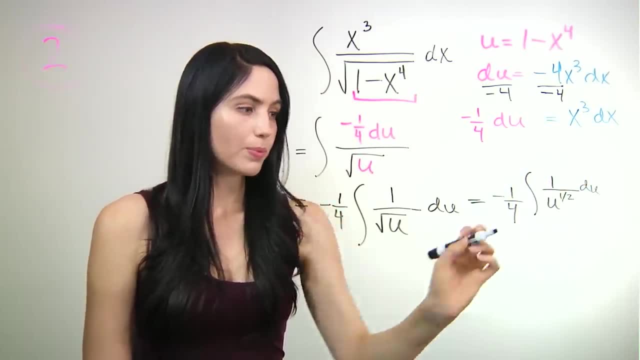 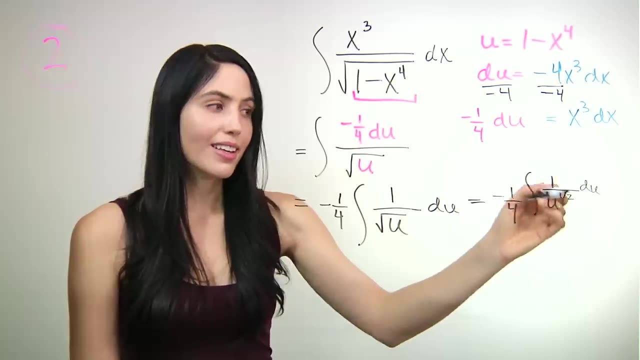 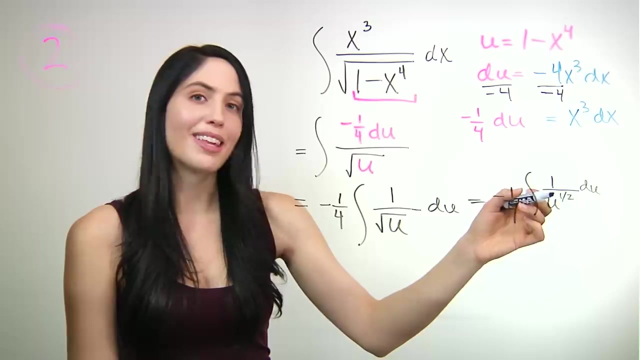 1 half power du. Now, since you know how to take the integral of a power, most likely what we want to do is bring this fractional power up to the top. When you bring a power up to the top of a fraction, you have to make: 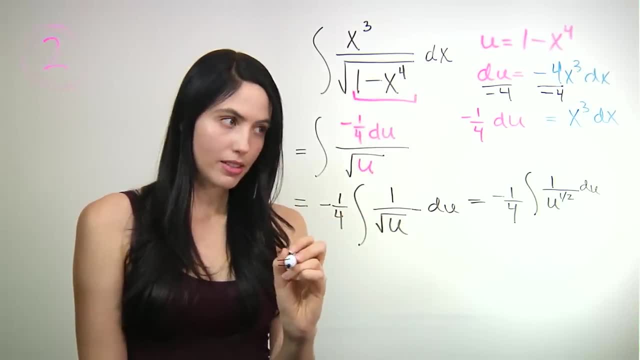 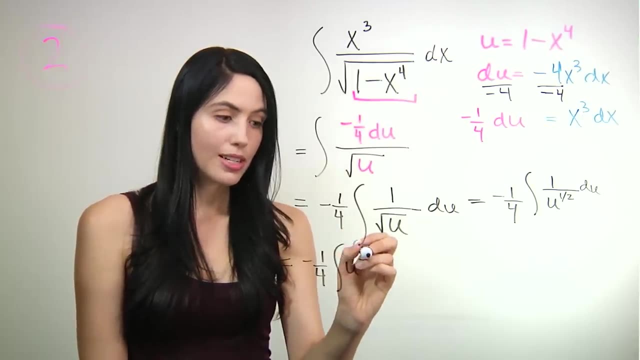 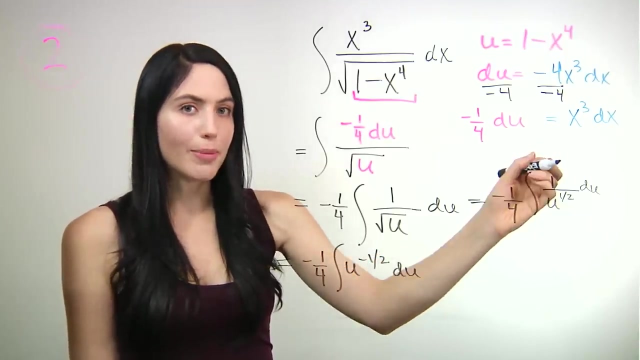 the power negative. So what you have is negative 1 fourth integral of u to the negative 1 half power du. Just remember: when you bring a power up to the top of the fraction it becomes negative. This negative power means 1 over. 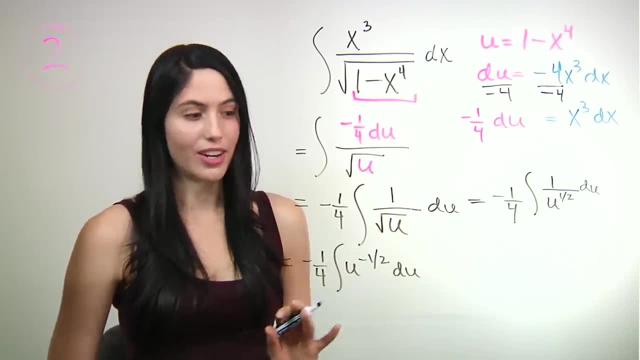 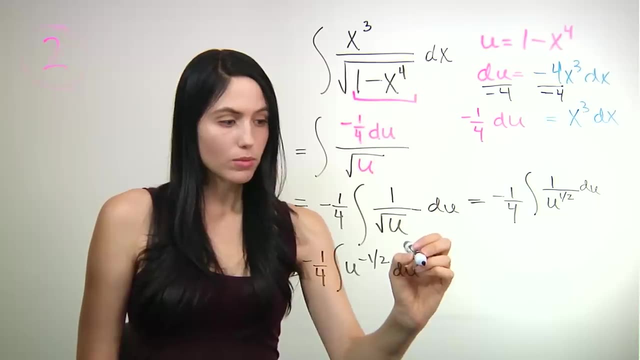 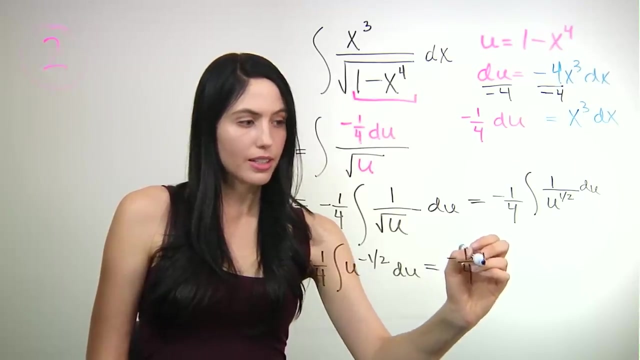 u to the 1 half power. Anyway, now you're really ready to integrate. All that work of doing u substitution was so that you can get to this point and integrate. So when you integrate that, you get negative 1. fourth and you're going. 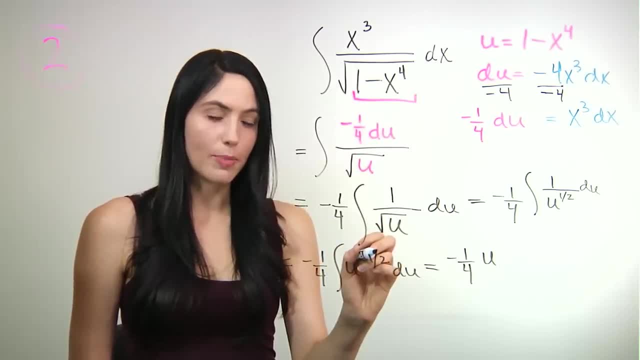 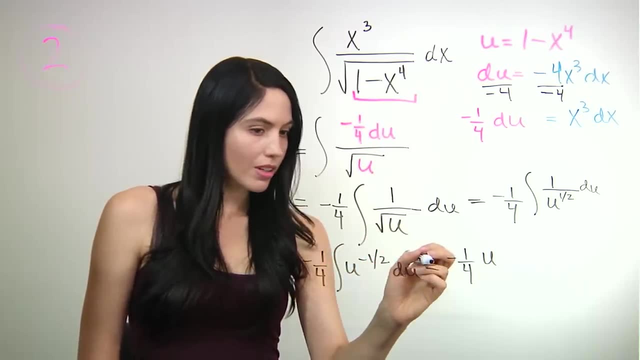 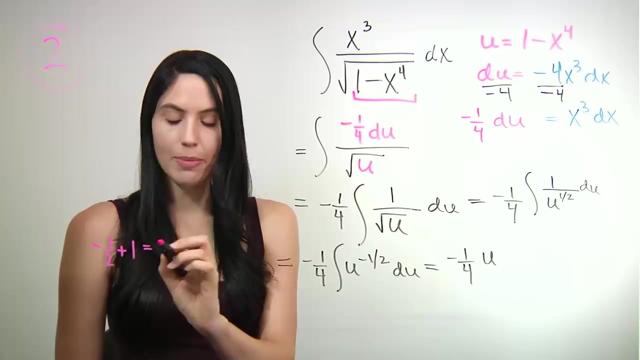 to raise the power by 1.. This is the power rule. When you add 1 to negative 1 half, when you add 1 to negative 1 half, it's the same as adding 2 over 2. So you end up. 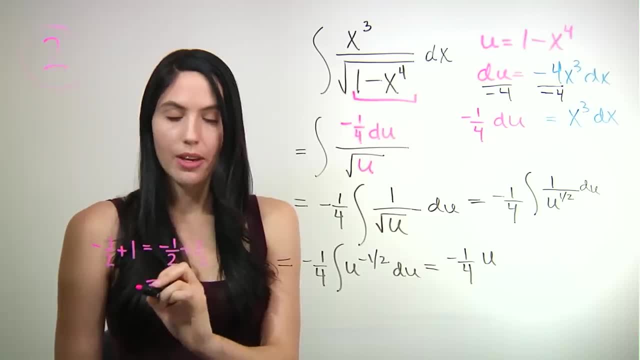 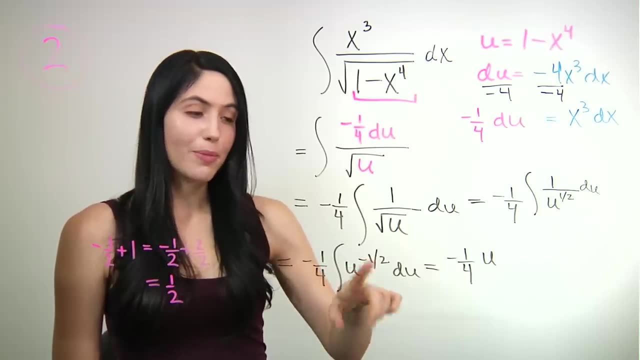 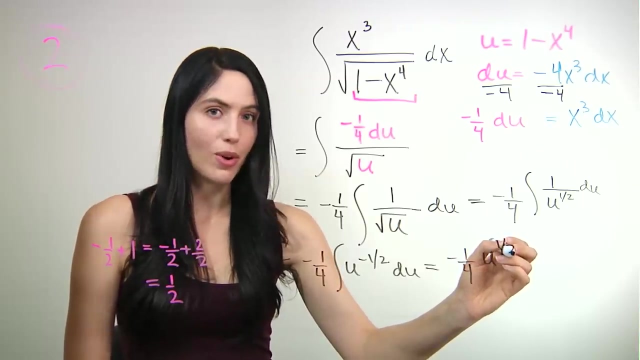 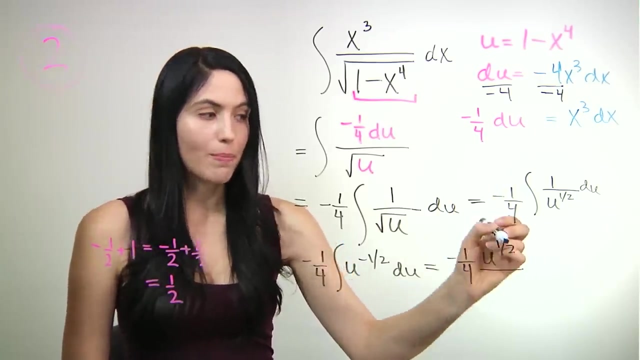 with positive 1 half. Anyway, when you raise u to the negative 1 half power, you get u to the positive 1 half power. Then, by the power rule, you need to divide by the power you just raised it to. 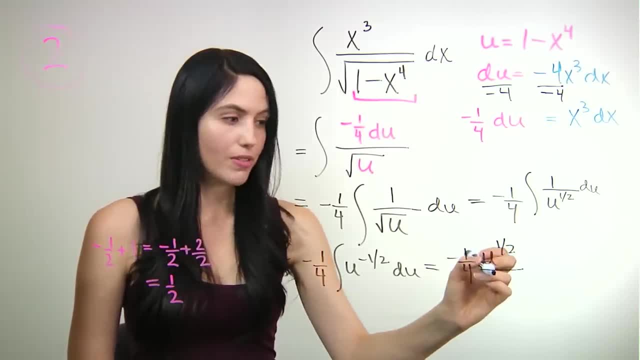 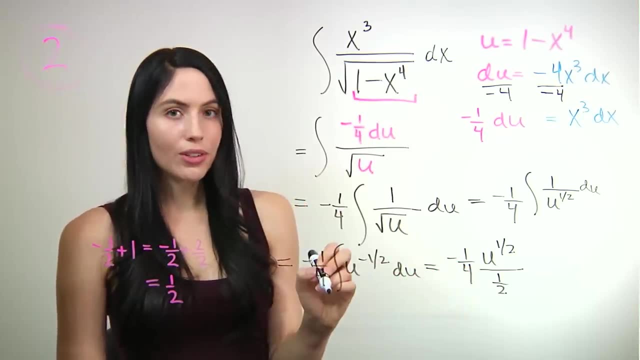 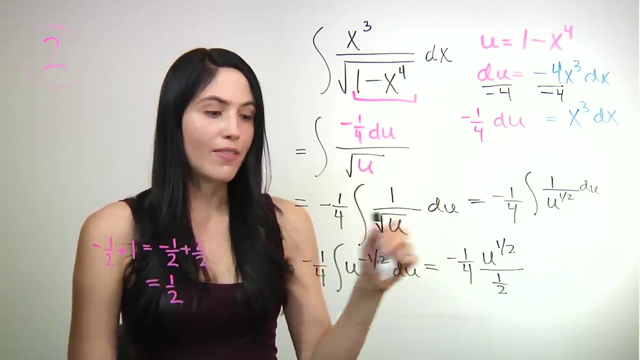 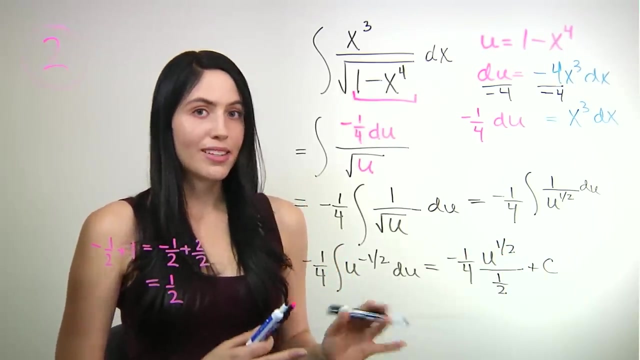 the number you just raised it to. So you divide by 1 half. Now, when the integral goes away, when you integrate, when this integral symbol goes away, and since it's indefinite, no limit, you must write plus c, Don't. 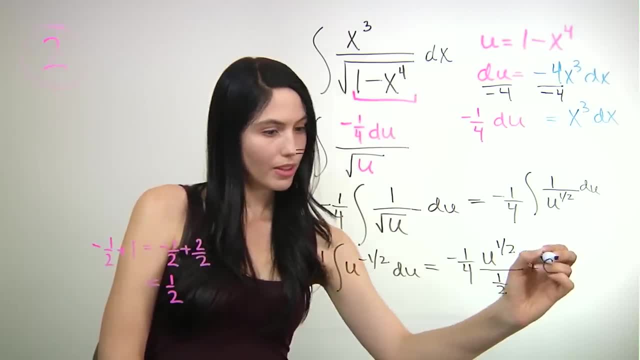 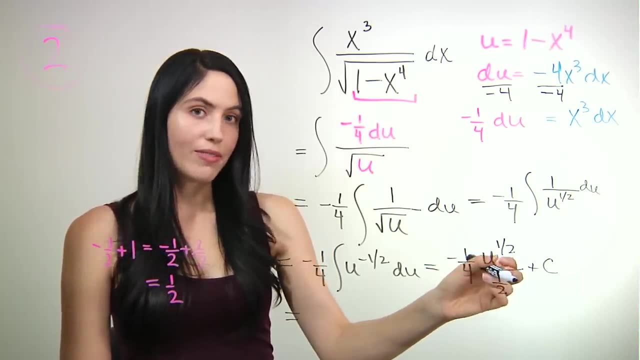 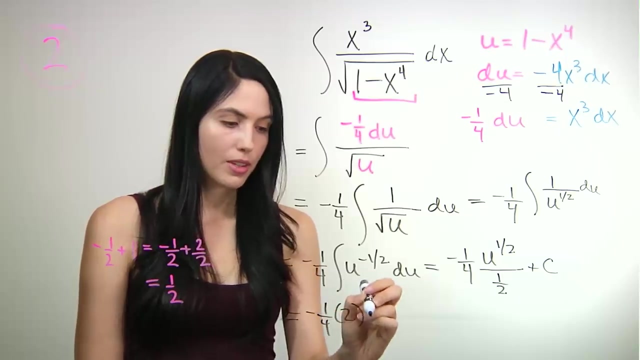 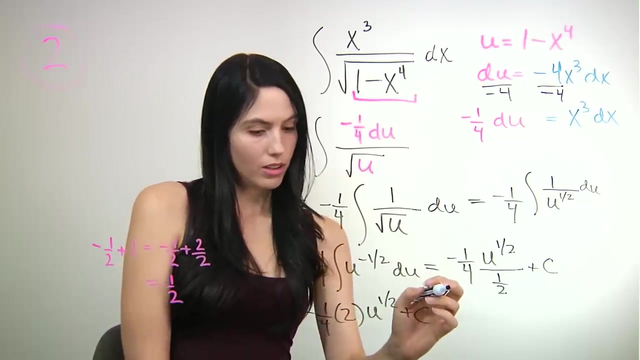 forget that. Now do some basic simplifying. And you have, because you're dividing by 1 half. it's the same as multiplying by 2. So you get 1 half plus c And that simplifies to negative 1 half. 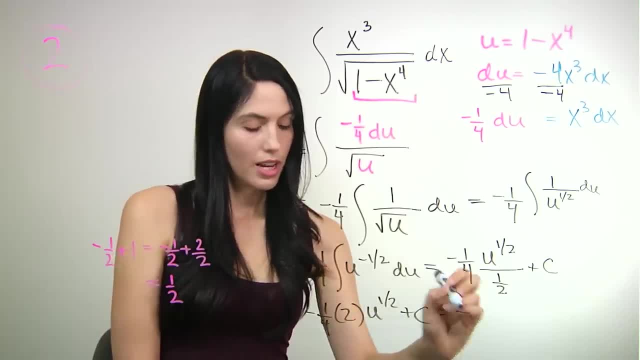 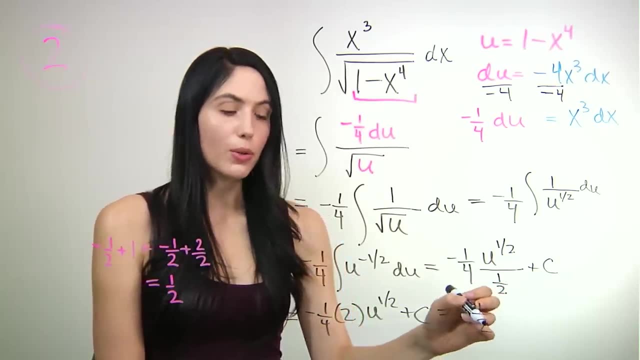 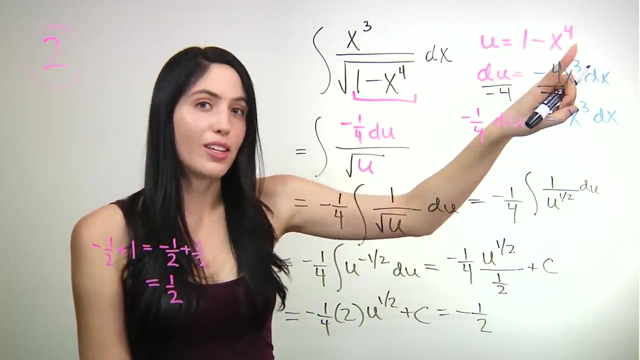 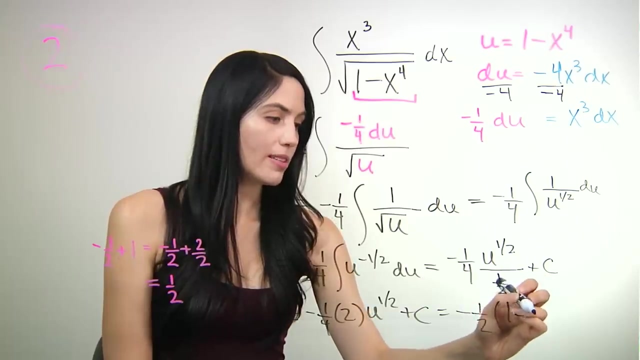 But in place of u, remember you need to back substitute, put back the original x expression that you set u equal to. So in place of u, you're going to write 1 minus x to the 4th. That is all raised. 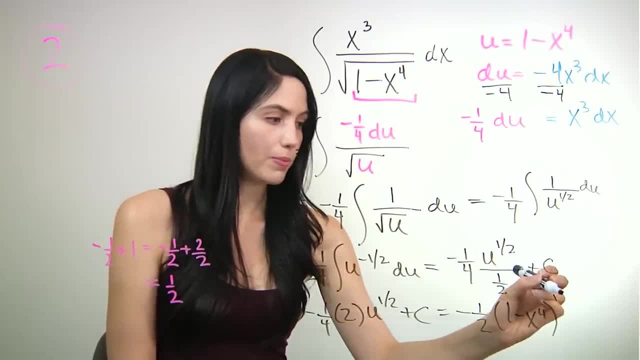 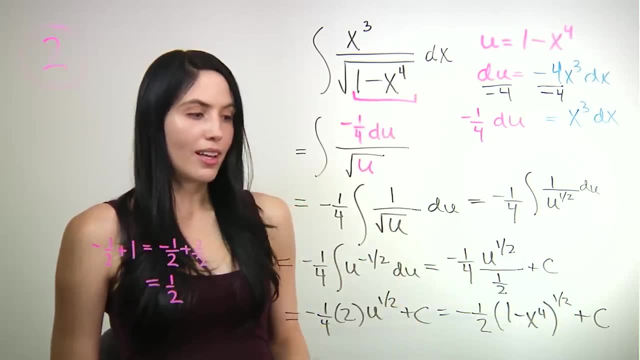 all of that is raised to the positive 1 half power and plus c. You might wonder why the c doesn't have a negative 1 half. even if you did multiply the c by negative 1 fourth, It wouldn't matter because c 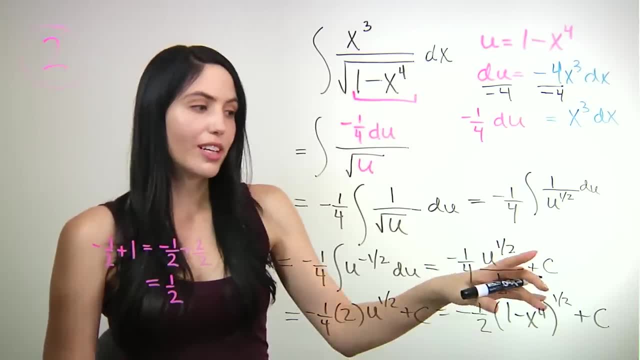 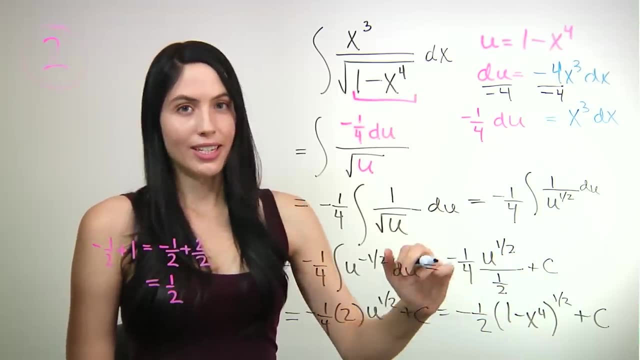 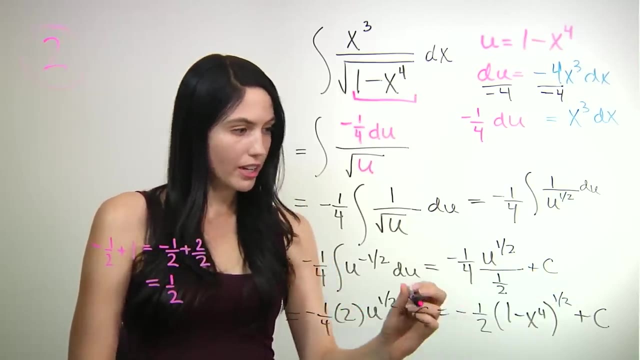 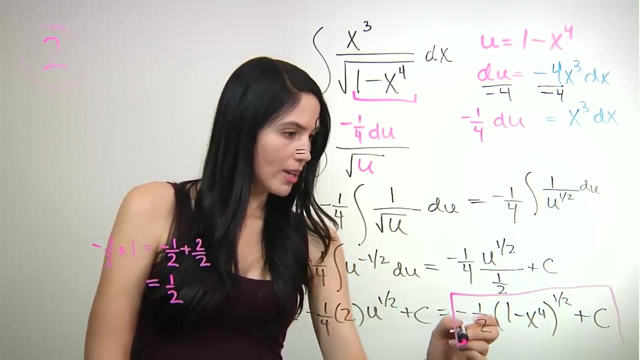 right now doesn't have any meaning. It doesn't have any value. We don't know what it is yet. It's an indefinite integral. So even if you change c, you could still get. the answer, for this integral is negative 1 half. 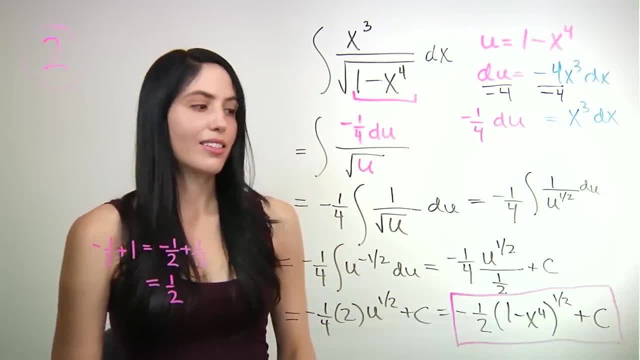 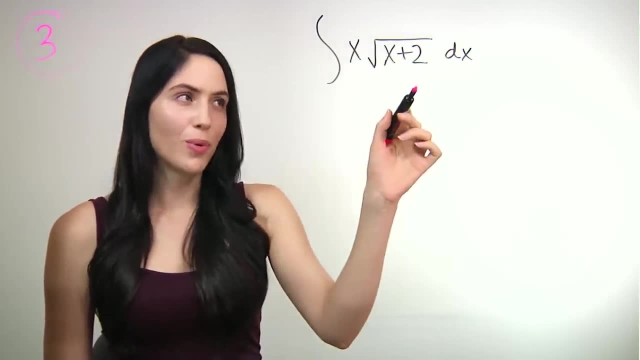 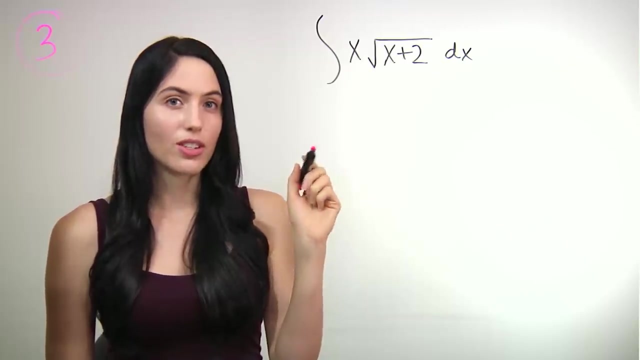 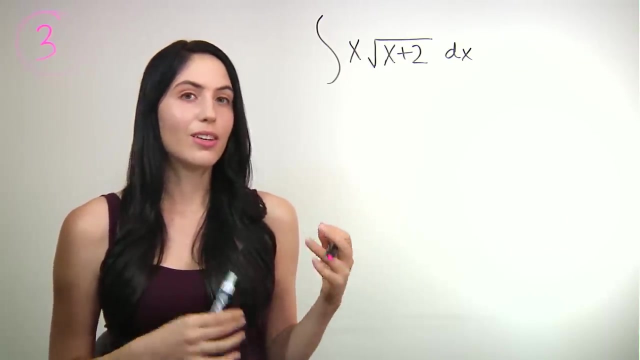 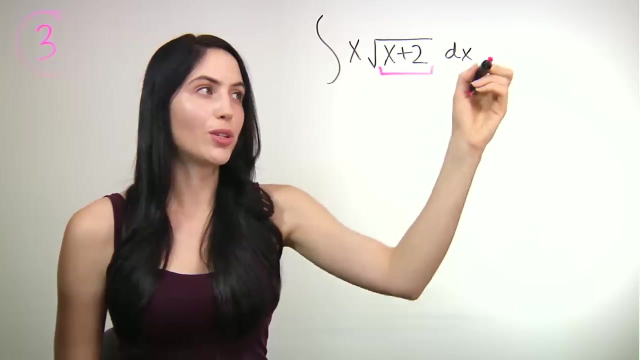 times 1 minus x to the 4th, raised to the 1 half power plus c And you're done. Okay, here's another one where the u is inside something, So you can use the radical to pick your u expression Pick. 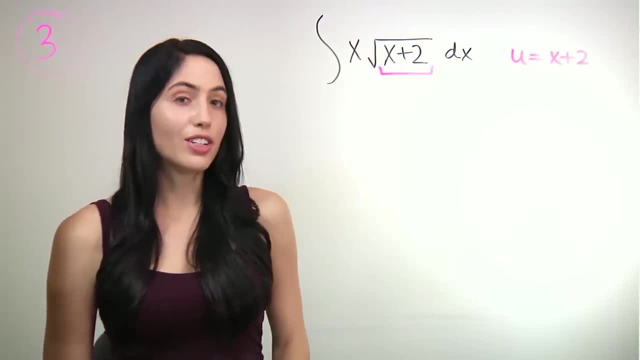 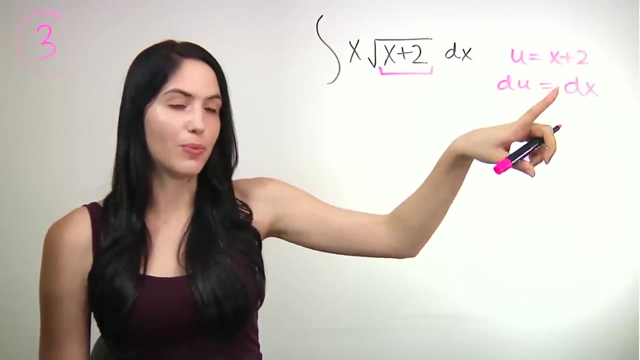 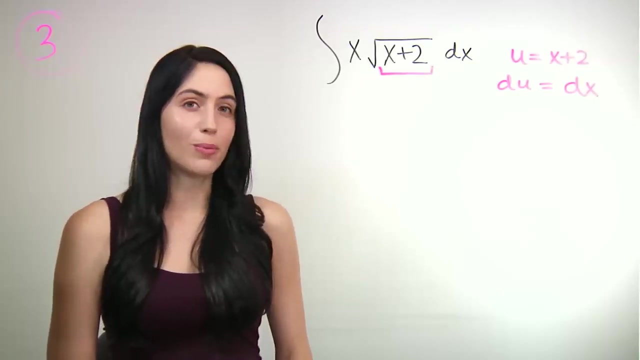 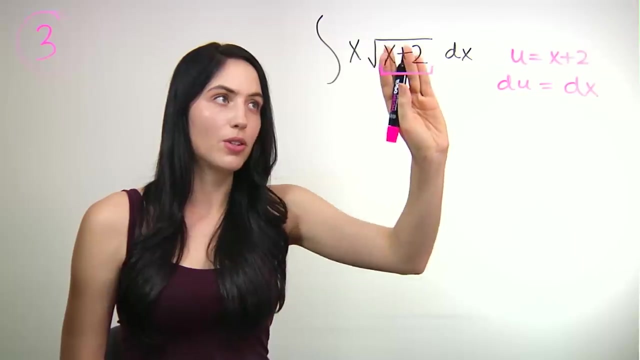 wisely. The best choice is usually the longer x expression that's inside something So good if you can just write dx, Now check to see if you can replace everything in terms of u and du. That's always your goal in u substitution. 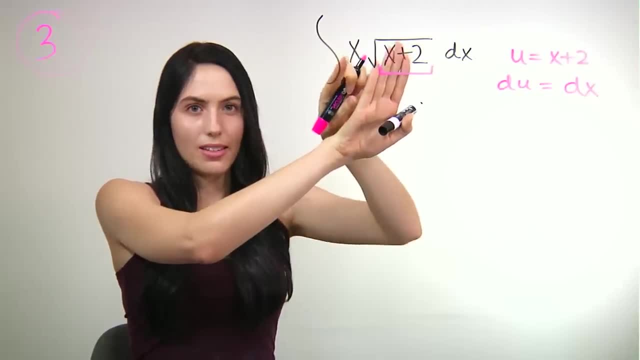 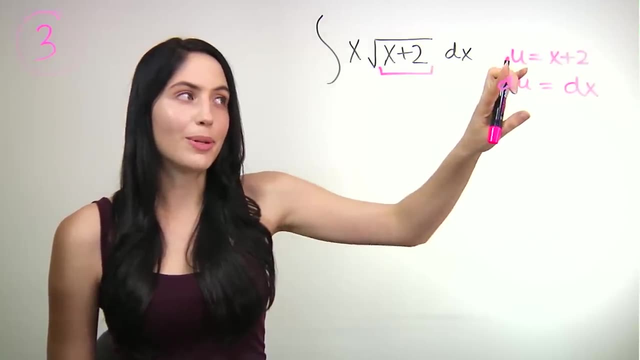 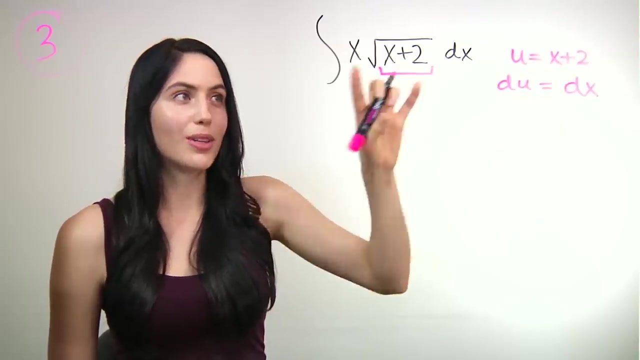 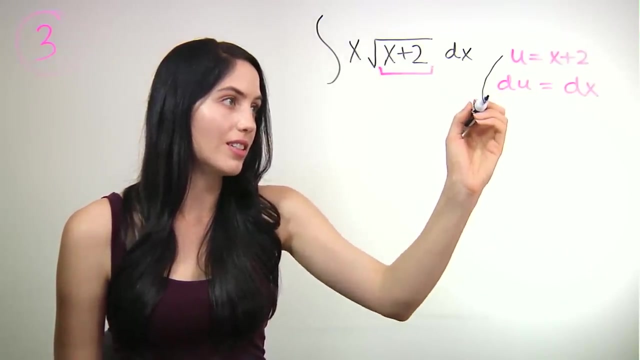 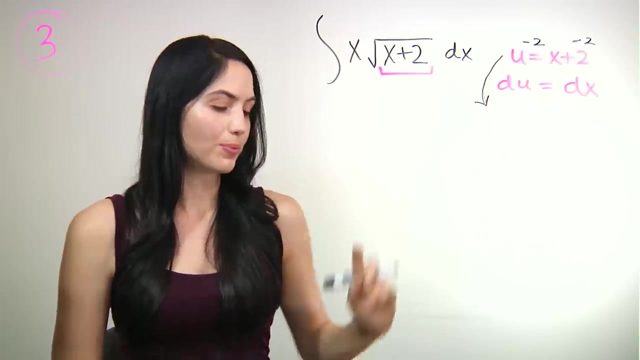 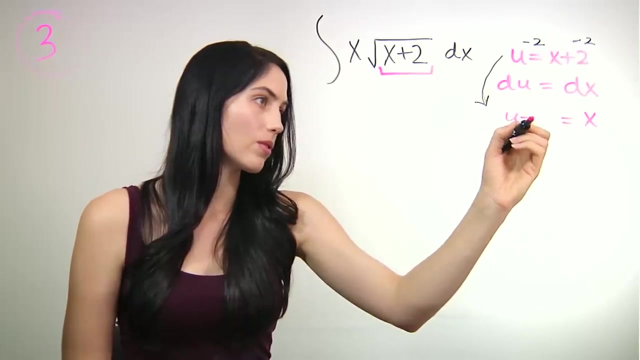 You can replace this with u Here. this is your u expression, So you want to rearrange it somehow to get x alone. So you want to rearrange that expression. Do it down here: You can subtract 2 from x, So. 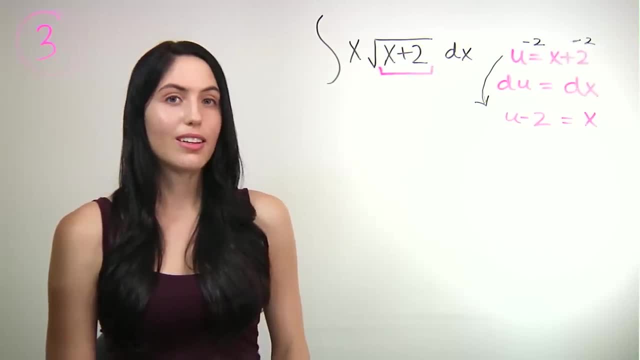 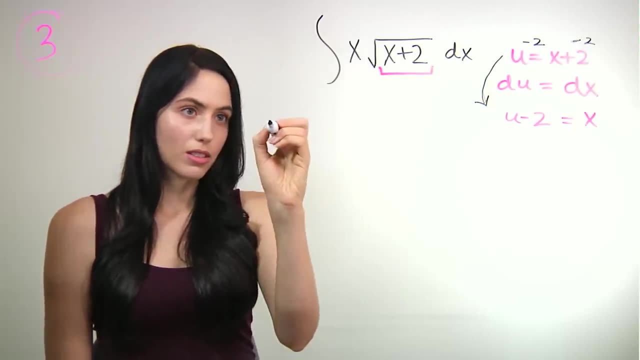 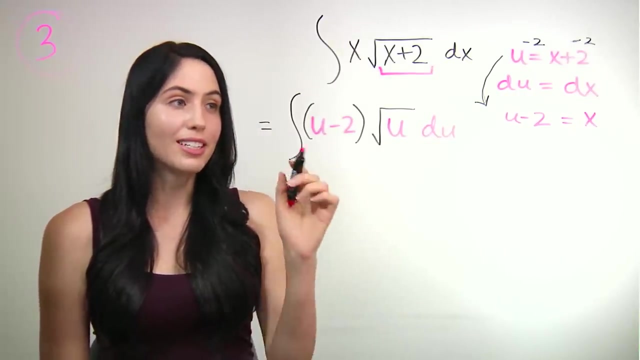 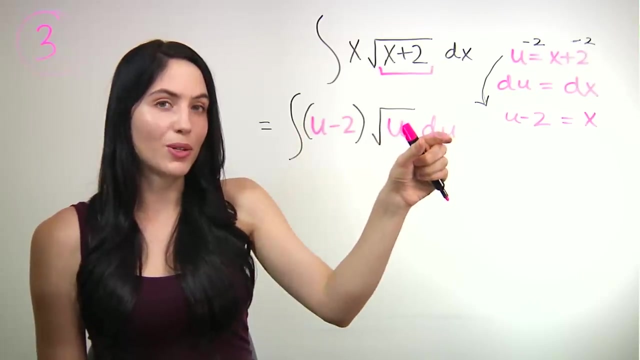 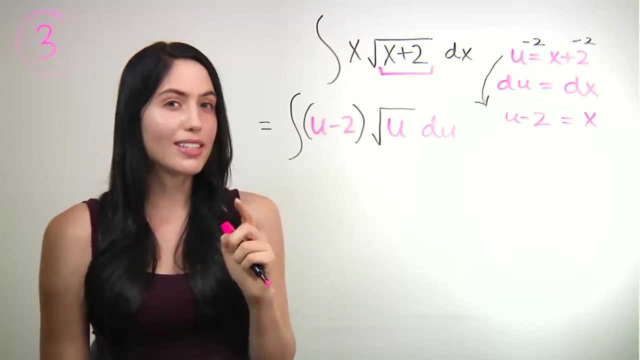 that gives you: x equals u minus 2.. Now you can substitute everything to be in terms of u and du. So now you've plugged in u minus 2 for x. So now everything is in terms of u and du. 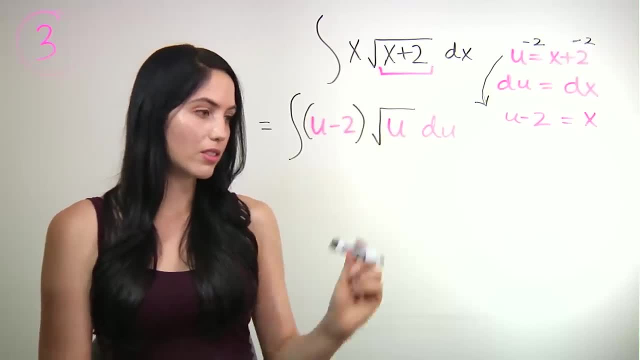 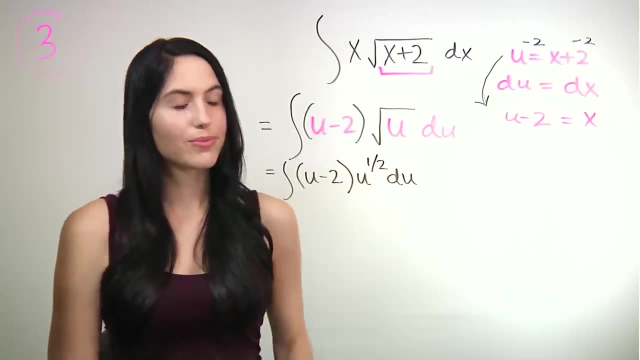 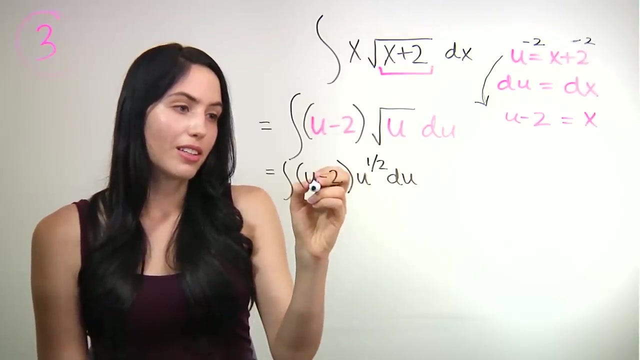 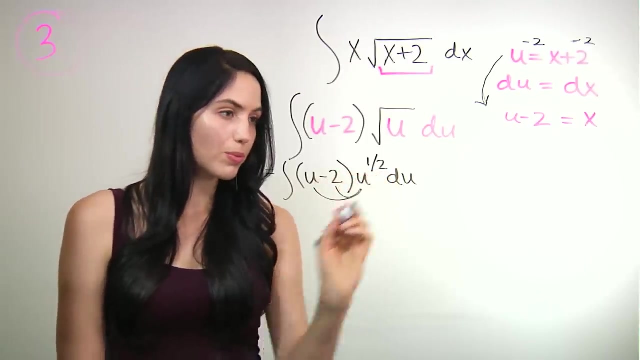 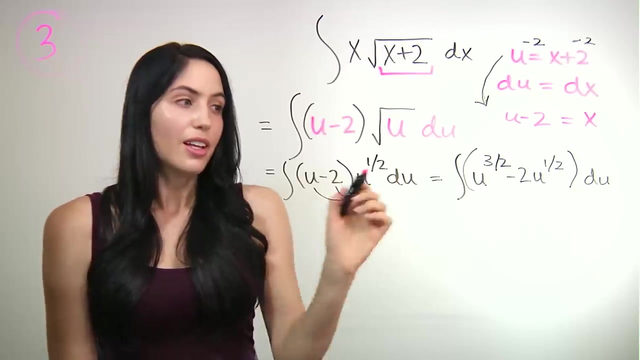 so you can integrate. It will be easier for you to rewrite this root as a power of 1 half. It will also make it easier if you multiply this by 1 half. So that gives you this power is 3 halves, because this was. 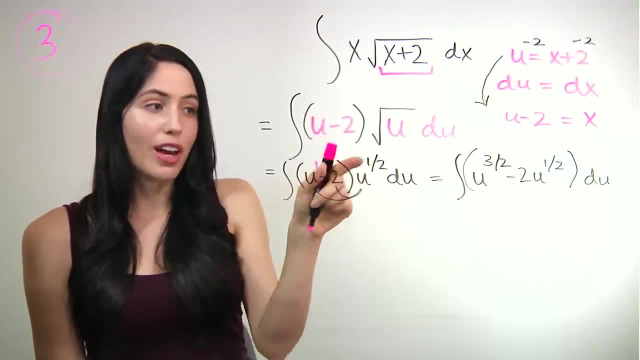 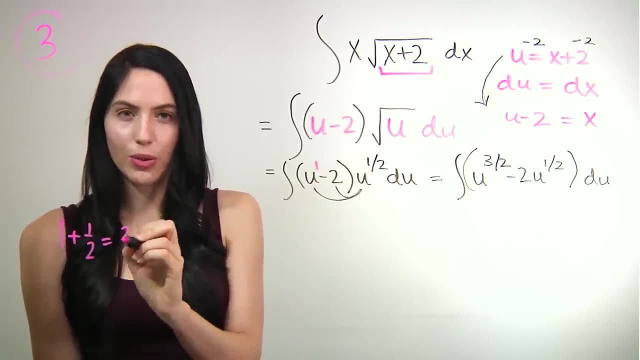 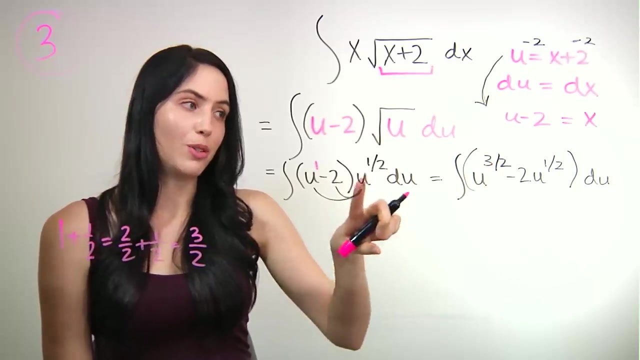 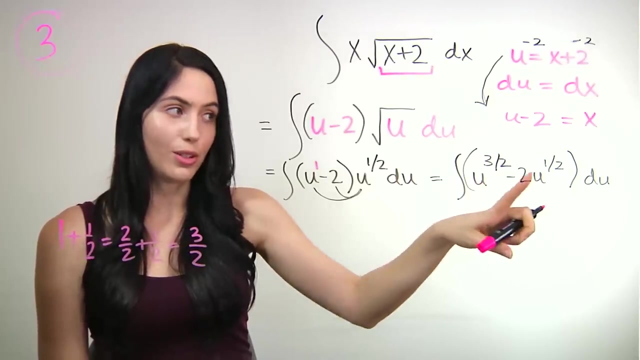 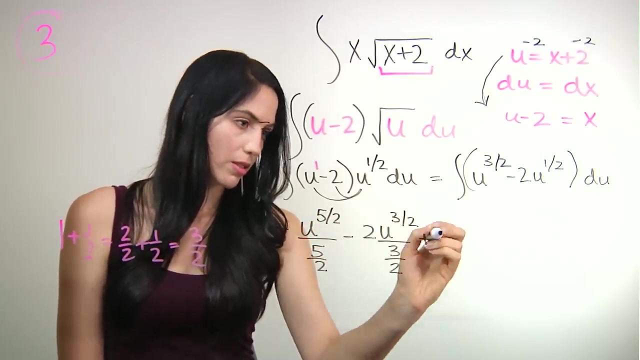 u to the first times? u to the 1 half. What you have to do is add those exponents. So this is 3 halves and this is just minus 2? u to the 1 half power. Now you're actually ready to integrate. 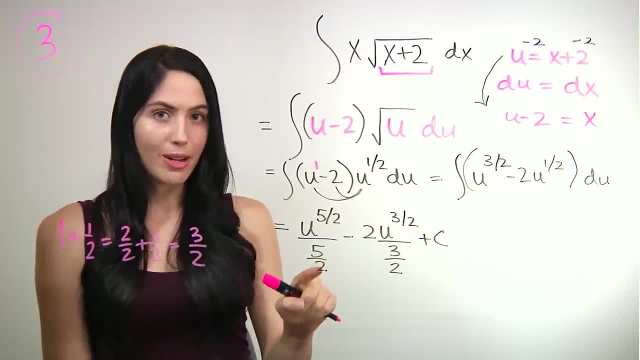 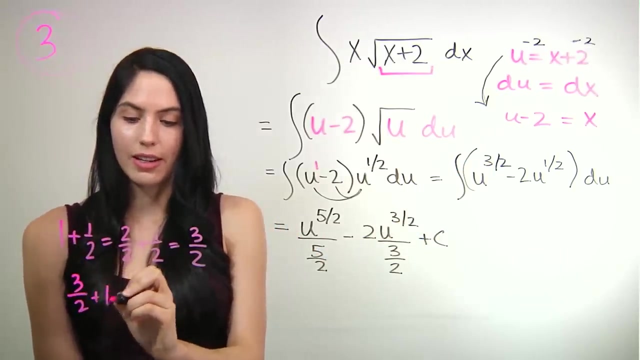 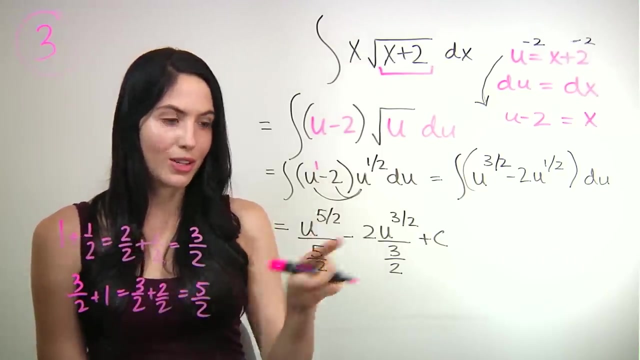 and you can use the power rule to integrate these two terms. Why is it 5 halves? Because 3 halves plus 1. if you do that math and get a common denominator is 3 halves plus 2 halves, which is 5 halves. 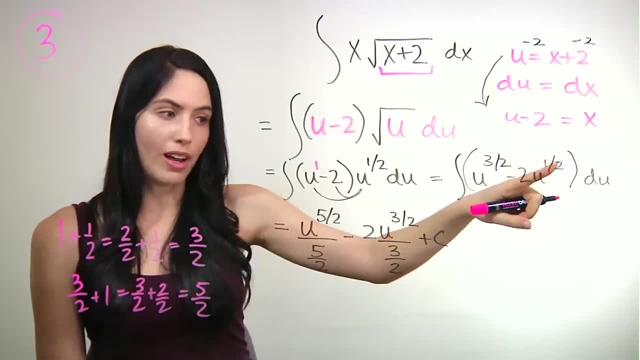 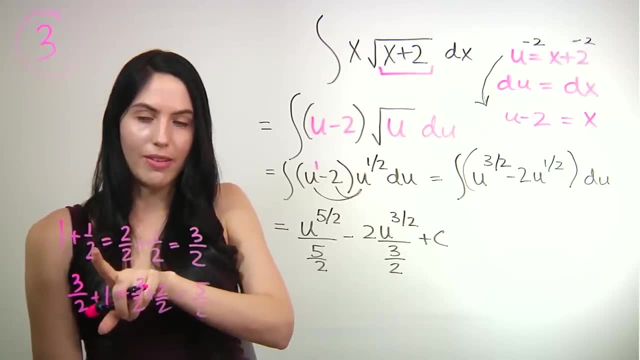 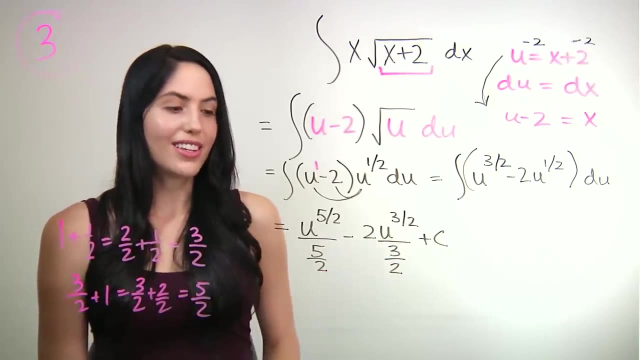 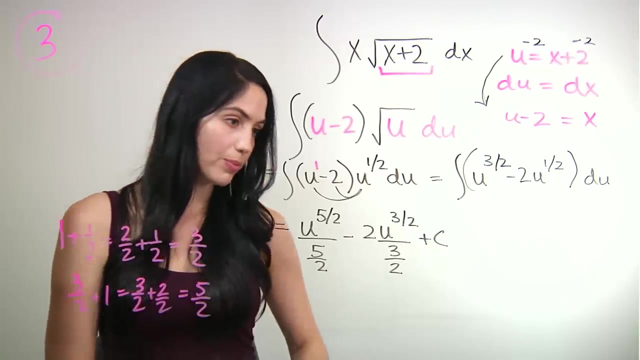 5 halves and you divide by the mu of power. Same thing for u to 1 is 1 half plus 2 halves, which is 3 halves and divided by 3 halves. OK, you can simplify this, because dividing by a fraction is the. 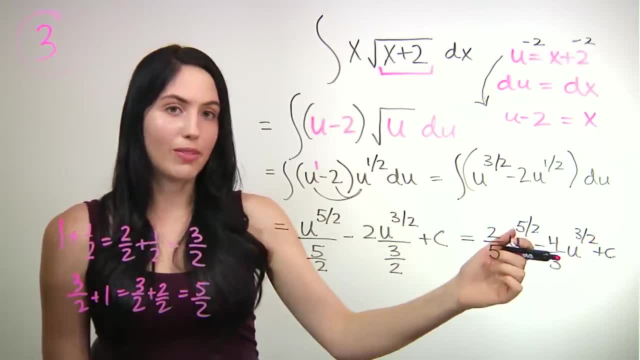 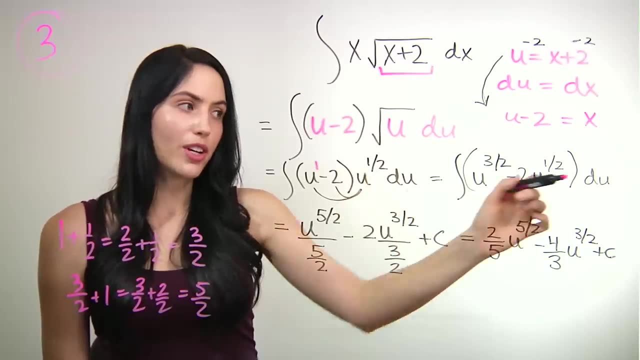 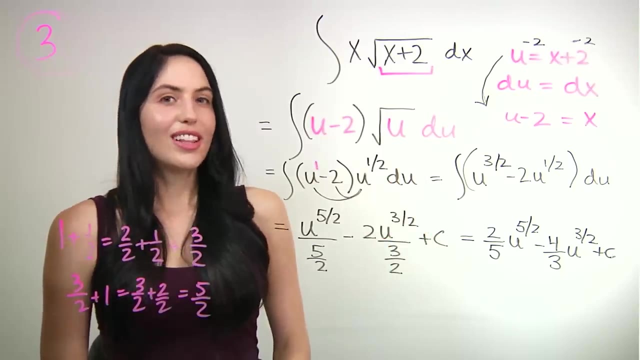 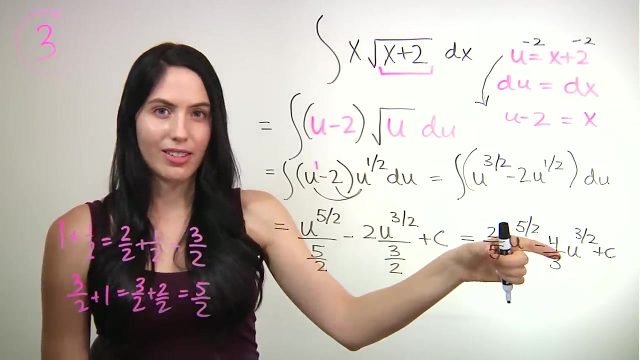 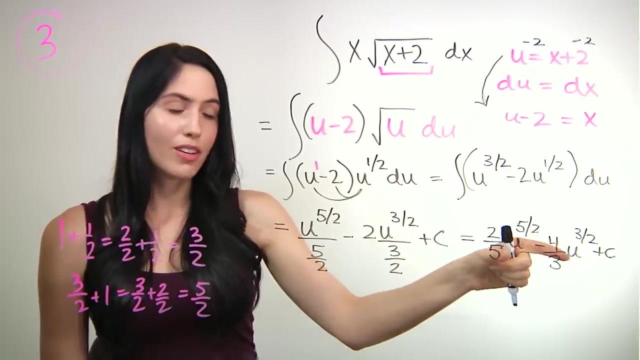 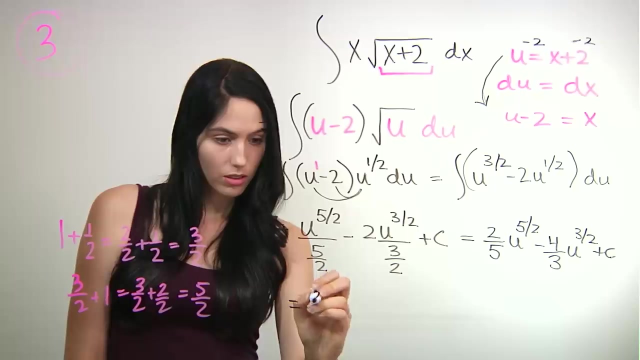 same as multiplying by its reciprocal, And this is what you get when you integrate and get rid of the integral symbol. The du goes away. Alright, there's one more step, which is to back substitute for u. You don't want to do this. 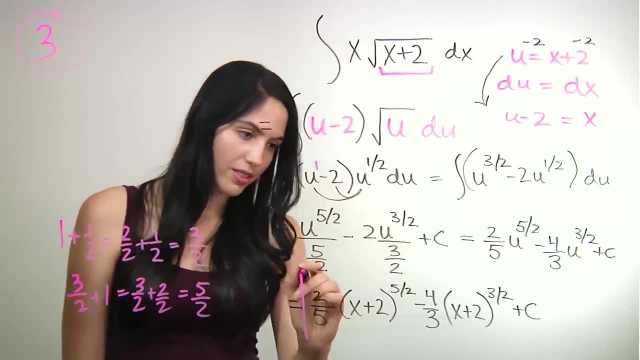 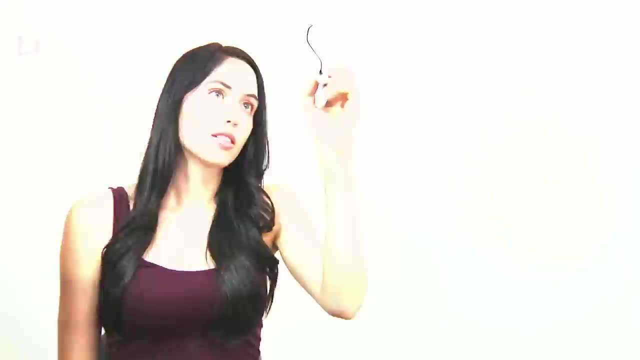 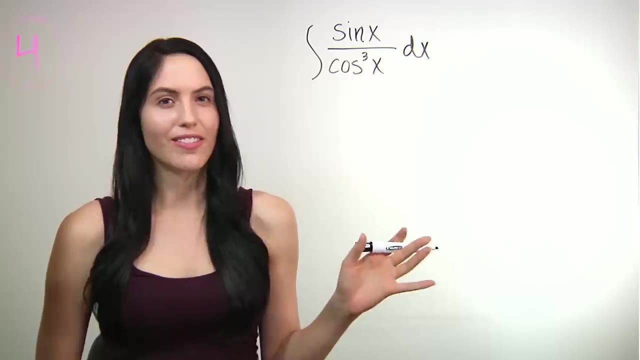 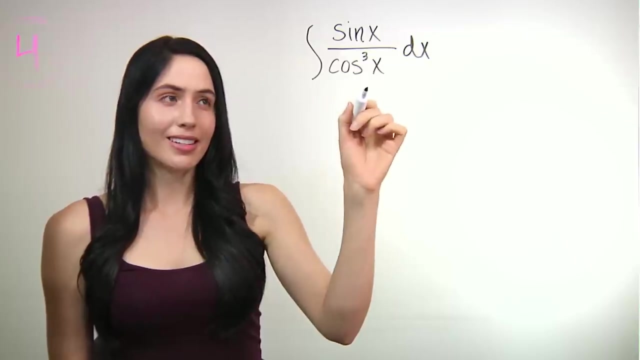 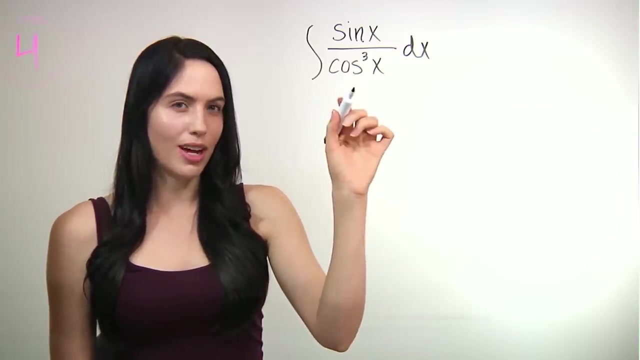 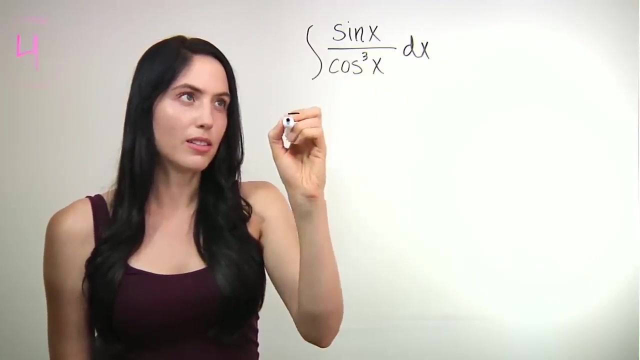 And you don't want to do this. So you want to add the integral to u And this is your final answer. OK, so you've seen a lot of the trig function. It's much easier to see what to do next if you rewrite. 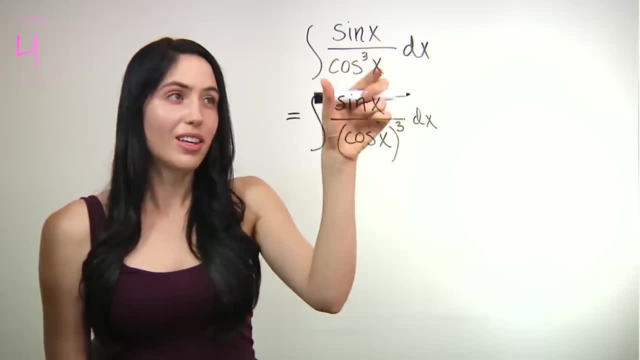 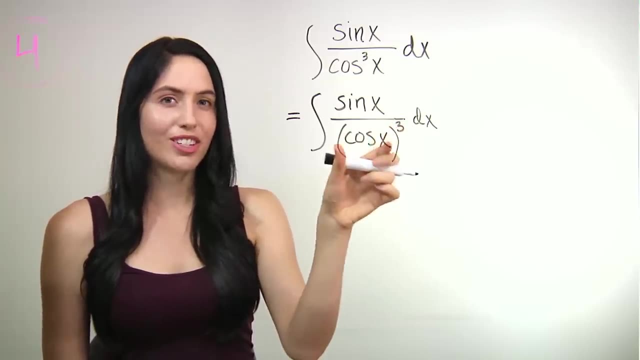 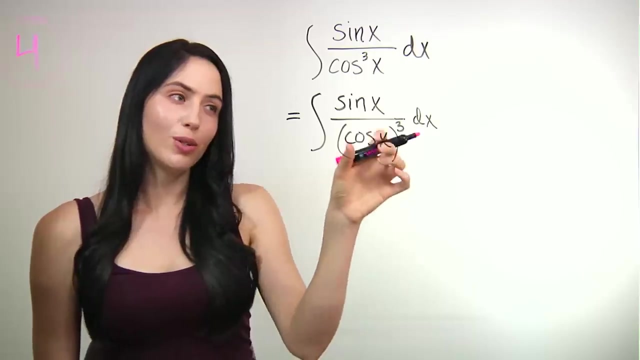 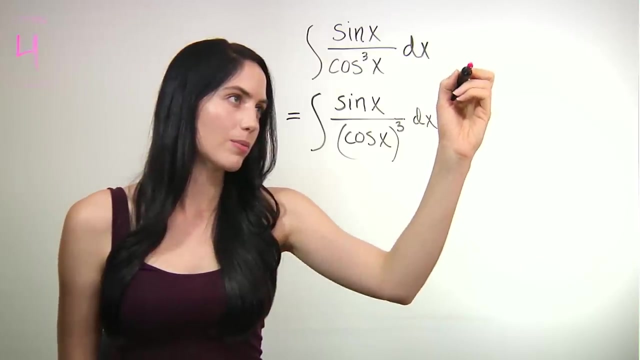 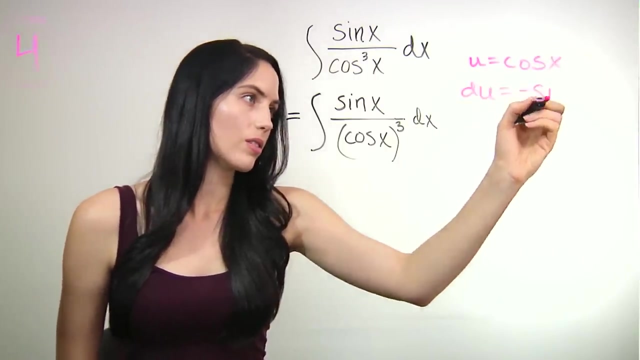 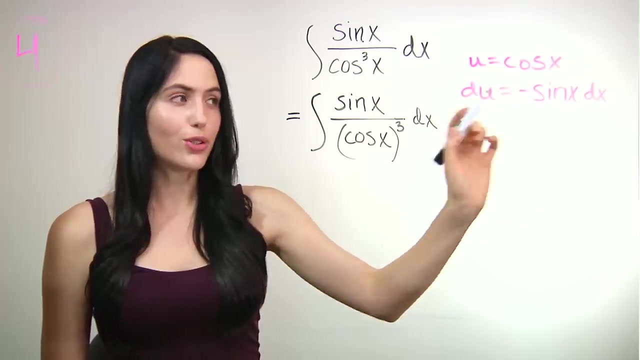 this with parentheses. This is sort of silly notation. I know What that looks like- is the derivative of cosine x, And the best choice is usually what's inside the power, So u can be equal to cosine x. Now find your du differential. 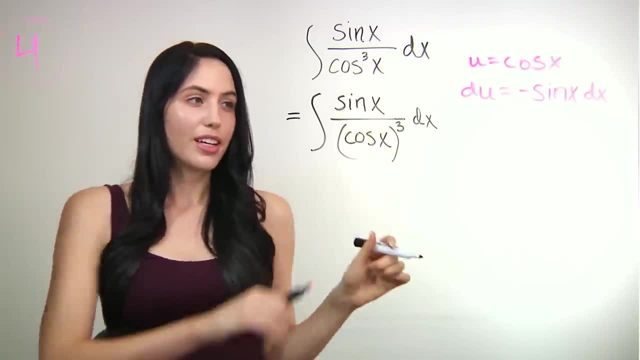 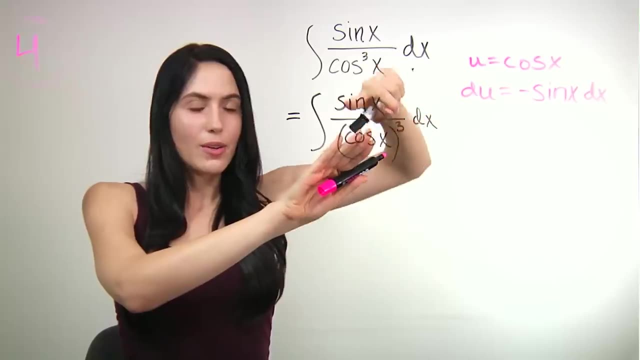 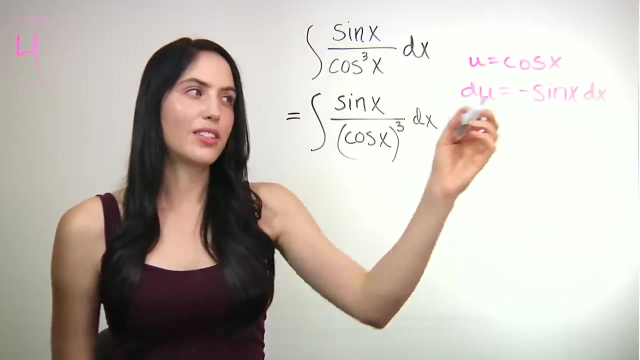 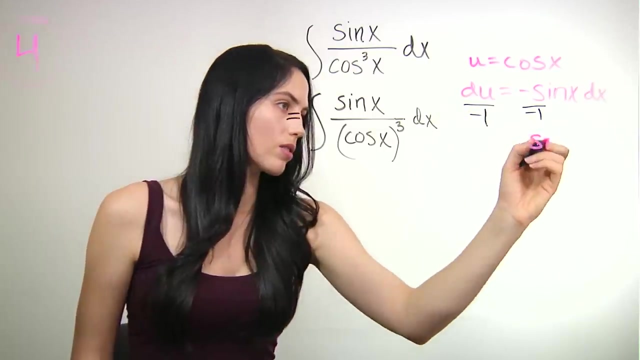 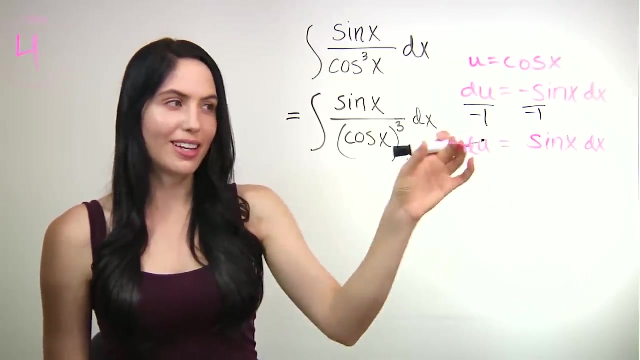 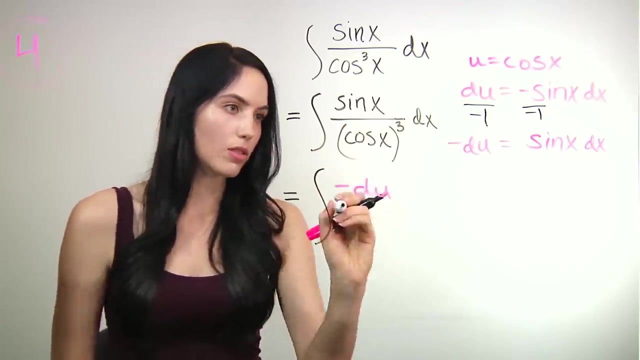 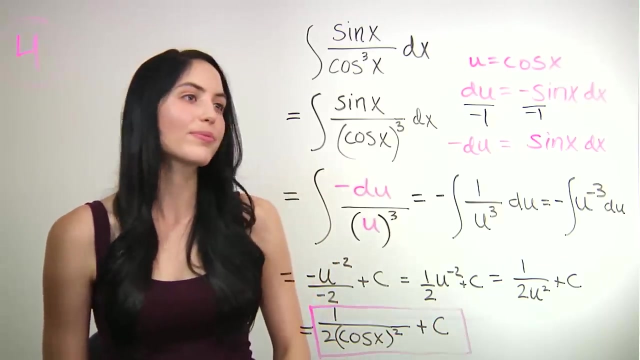 When you divide by negative sine x dx, you have positive sine x dx, So you're very close with just a negative sine difference. All you need to do is sine x dx equals negative du. Now replace everything in terms of u and du and integrate. 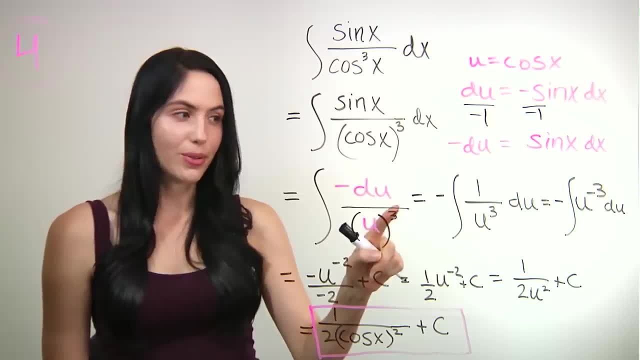 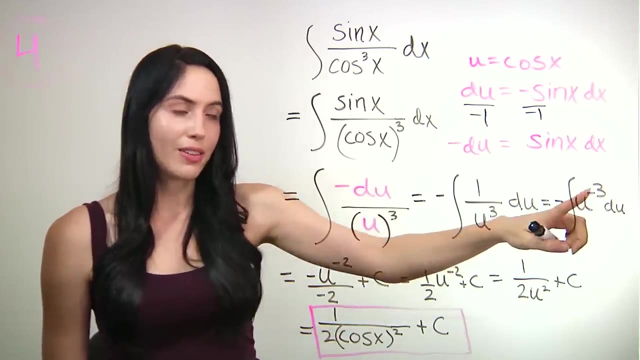 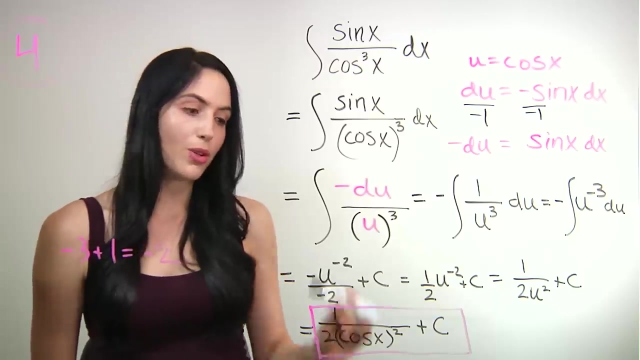 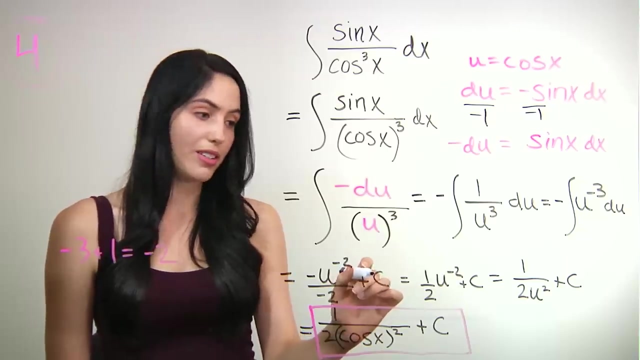 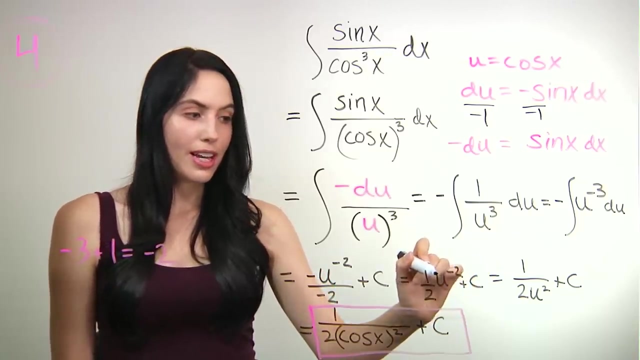 Okay. So when you replace everything in terms of u and du and du with the negative 3, power by 1 and divide by that new number, When you take negative 3 and raise it by 1,, add 1, you get negative. 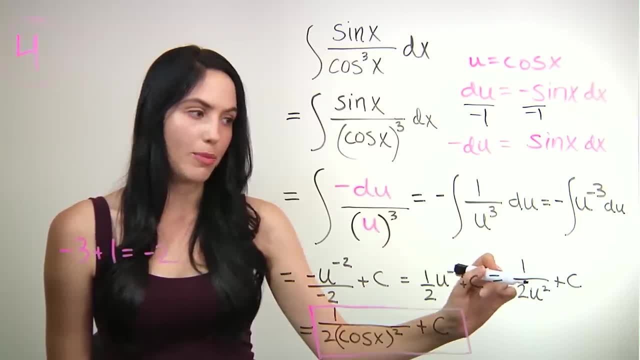 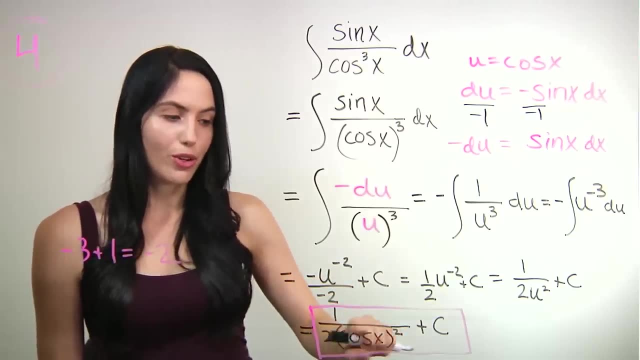 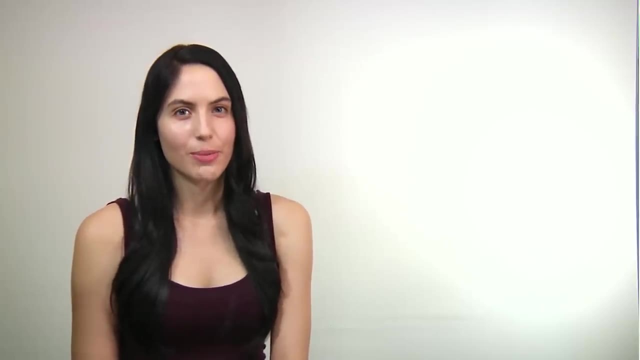 2 into a positive power by bringing it down into the denominator. So you have 1 over 2, u squared plus c, and then back substitute plug in cosine x for your u and that's your final answer. Thanks for watching, If you. have any questions, please leave a comment below. If you have any questions, please leave a comment below. If you have any questions, please write in. 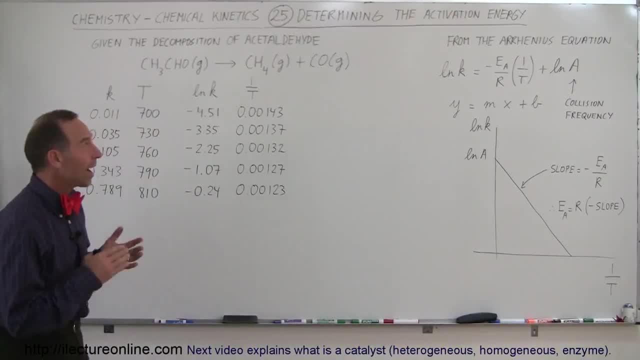 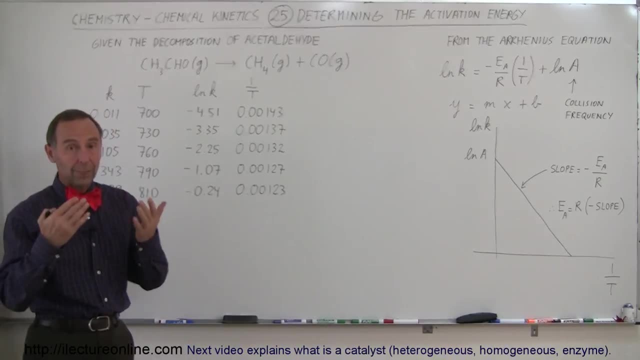 Welcome to Electron Line, and in this video we're going to show you how to find the activation energy of a reaction. Remember that the activation energy is something that a lot of reactions need, because not all collisions automatically end up in the molecules colliding, reacting with each other. Sometimes there 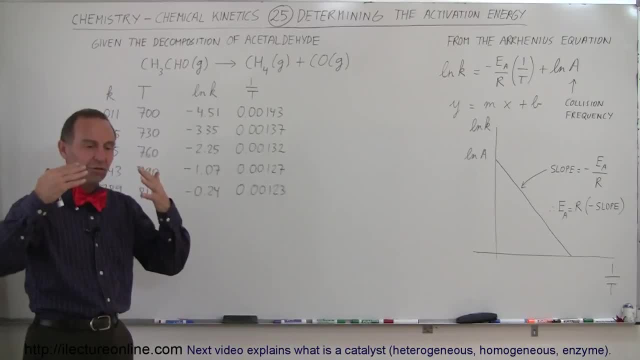 needs to be enough kinetic energy before the collision is violently enough so that the bonds in the molecules can be moved or bent or vibrated enough for the reaction action to take place. So how do we find that activation energy? Well, what we can do is we can take some measurements. So, for example, here we have: 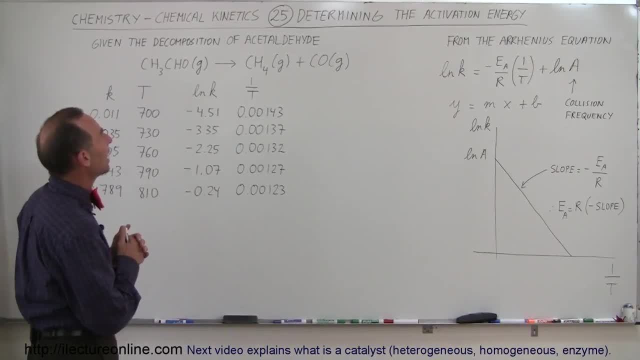 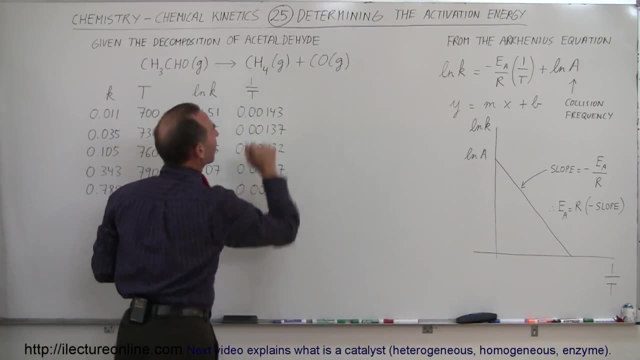 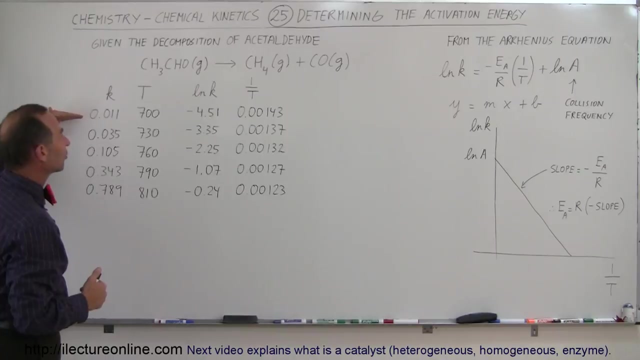 a sample decomposition of acetaldehyde. This is CH3CHO. it's a gas and it decomposes into methane and carbon monoxide gas. And let's say that we change the temperature and at various temperatures we measure the various reaction constants. And so, from the previous video, when we talked about the 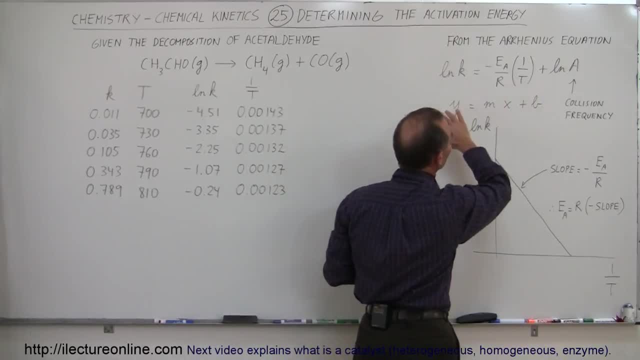 reaction constant. we measured the reaction constants, And so from the previous video, when we talked about the reaction constants, And so from the previous video when we talked about the Arrhenius equation, we saw that the equation had the form of a linear equation: y equals mx plus b, where the y was the natural log of the reaction. 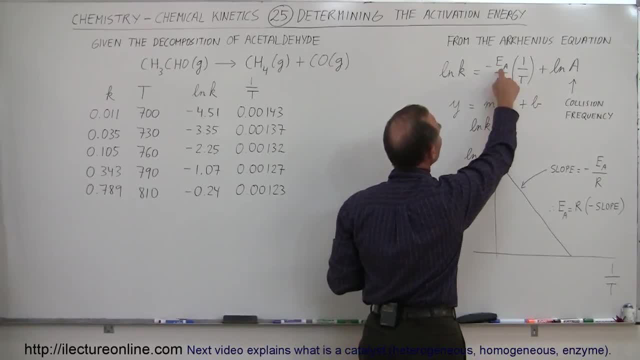 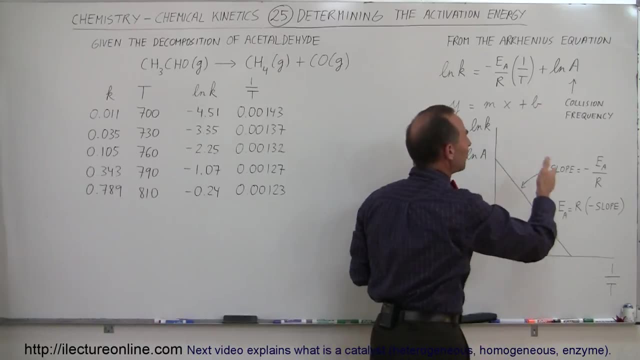 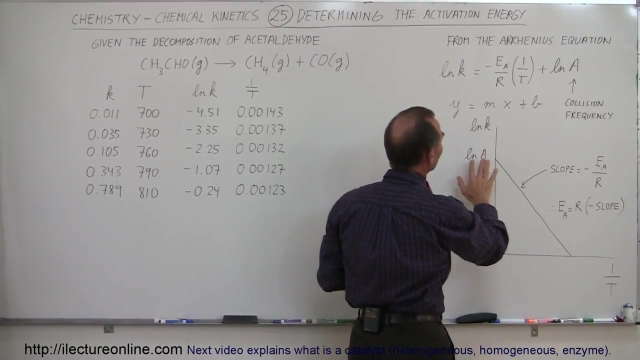 constants. The slope was the negative of the activation energy divided by the gas constant. x was 1 over the temperature and then b the, what we call the, where it crosses over the vertical axis. the intercept was the natural log of a, where a is what we call the collision frequency.